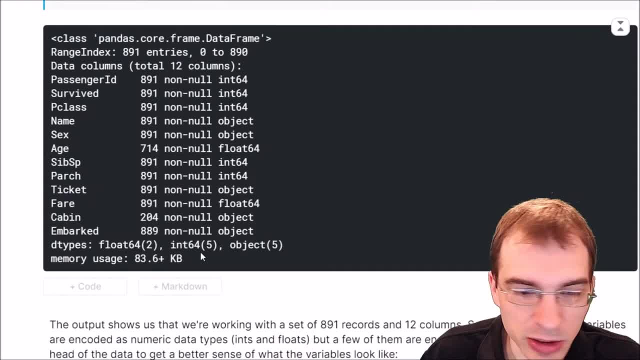 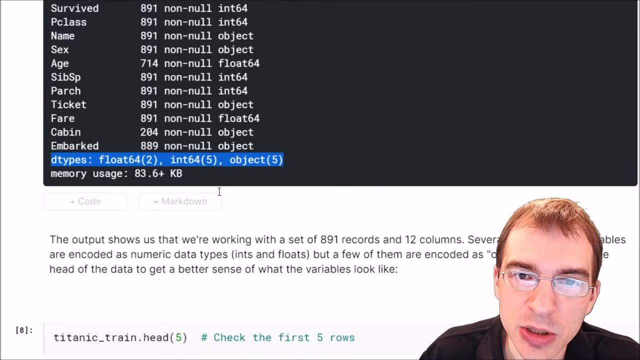 it contains and what types they are. So let's scroll down and look at the dot info output. We can see we have several data columns. There's 12 in total and we have 891 total records. Let's go ahead and look at some actual data entries or records by running dot head. So 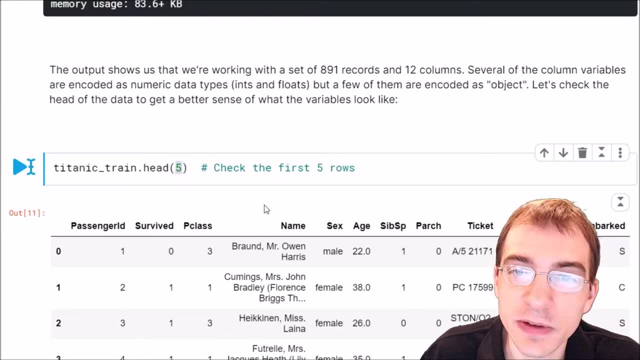 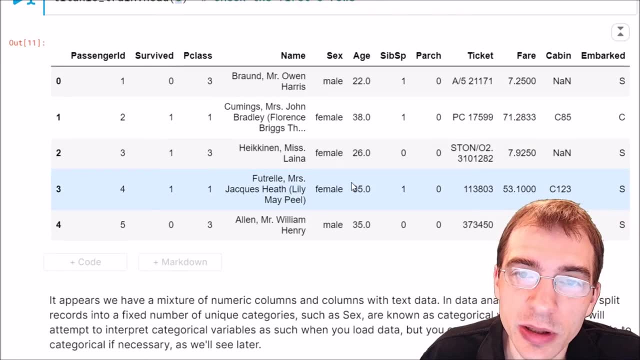 here we're going to run titanic train dot head. look at the first five entries and by inspecting some actual records we can get a better idea of what sorts of data we're working with and what it looks like like. so it looks like we have some passenger id survive. passenger class columns: the name of the. 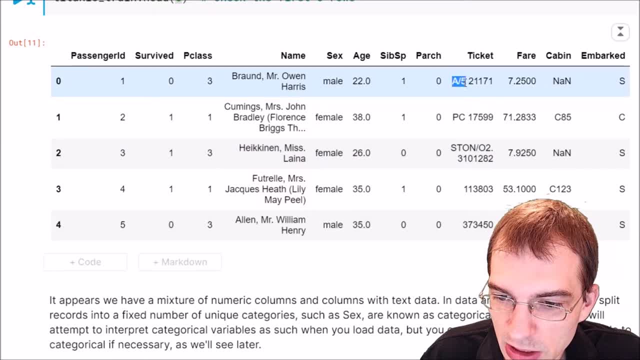 passenger, the fare that they paid their ticket and a cabin variable. i'm noticing right away, actually, that the cabin variable contains some- not a number- entries, so those are missing. so already we see that this data set is going to contain some missing values. we're probably going to have to 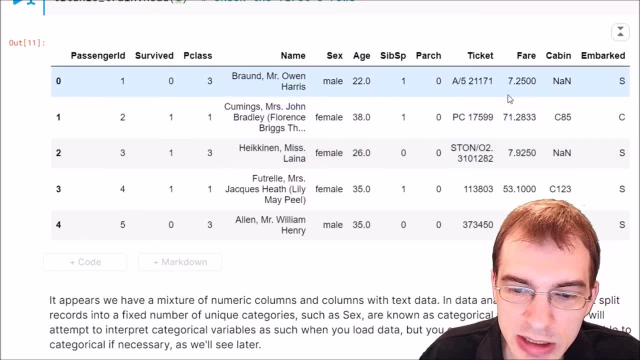 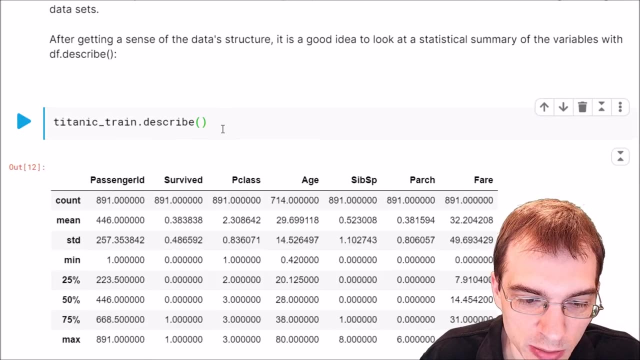 figure out how to deal with. so, after gaining some sense of the types of records we have, let's run another summary function, describe, to get an idea of the distribution of these numerical columns. so we'll scroll down here and run titanic train dot, describe. so this is pulling up summary. 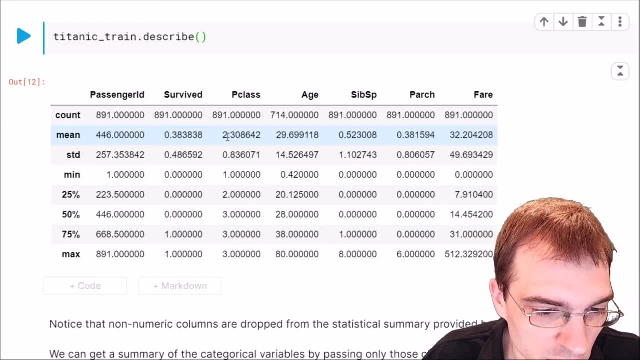 statistics on each of the numeric columns, so you can see here, for instance, passenger id. well, this just seems to be a number going from one to eight, ninety one, so we're going to go ahead and do that. so essentially, each row is just given a unique passenger id, so that's not particularly. 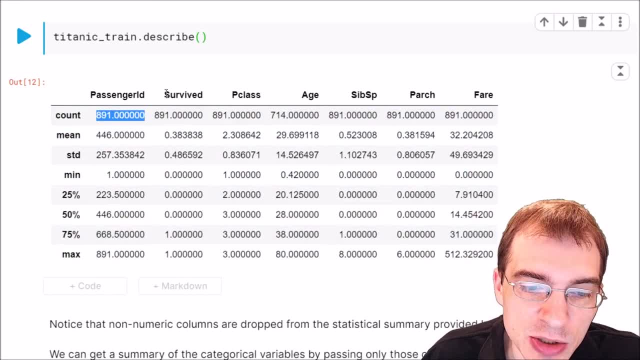 interesting for us. the column survived is actually the target for prediction for this competition, so this variable actually tells us whether a given passenger survived the titanic disaster or not. so that is actually one that's very important for us to look at. so let's see what that is. 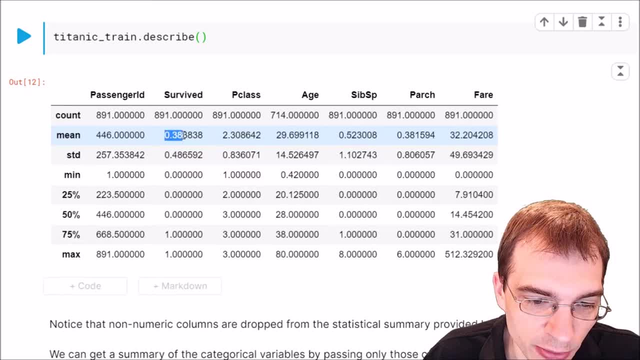 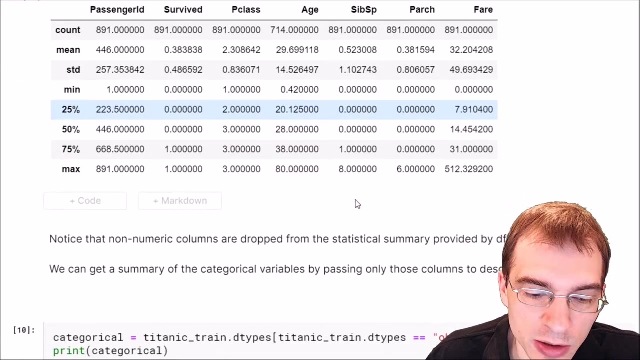 we can see, the average of survived is 0.38. that means that a approximately 38 of these passengers survived, which means most of them actually did not survive. now notice that when we ran describe, it only kept the numeric columns because it can't run summary statistics on categorical columns, so we'll look at those separately here. let's just 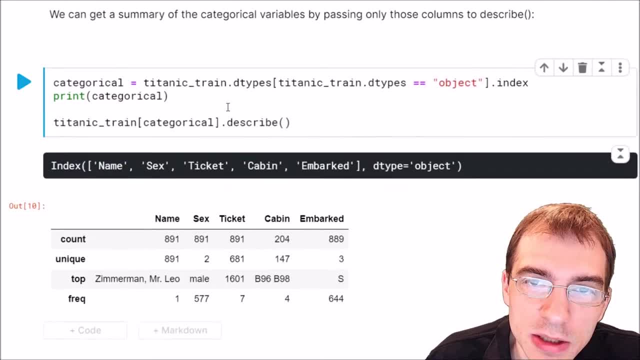 make a list of the columns that are categorical. so to do that, we're going to make a list of the categorical columns with this construction here. basically, all this is doing is saying we want to find the columns where the d type is an object, so that's. 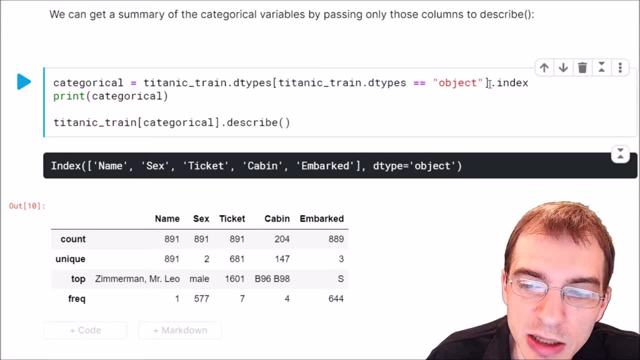 things other than numbers and we want to take the index of those columns and we'll save those as the categorical columns and then we're just going to use that, those column names, to index back into titanic train to get only the categorical columns, and then we'll rerun dot describe. but now 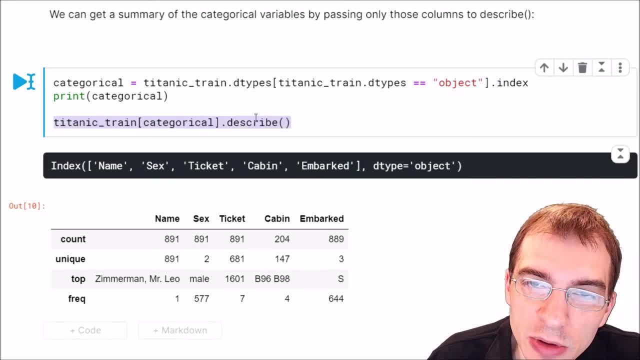 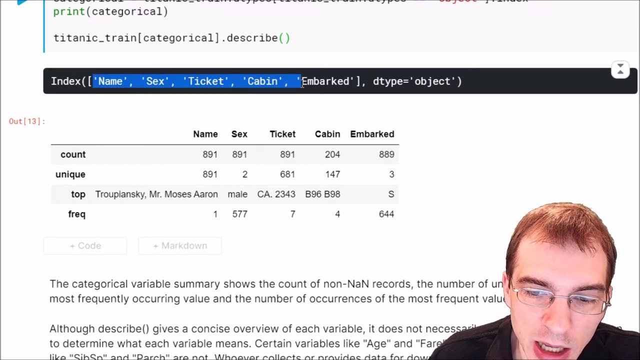 since we're only running it on categorical columns, it will run a different describe operation that works on categories instead of the one that works on numeric columns. So let's run this and just see what the result is. We can see. these are the categorical columns. name: sex ticket cabin embarked. 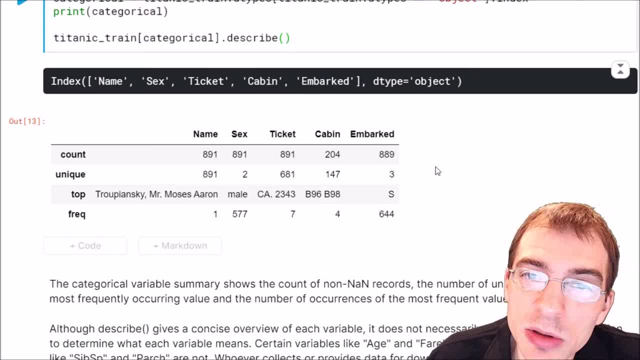 And when we run describe on this, it just gives us a table showing the count of each column, the number of unique different entries for each column, the top most frequently seen entry and the frequency of the most seen entry. So, for instance, under the sex column, it's showing us that there are two unique values. 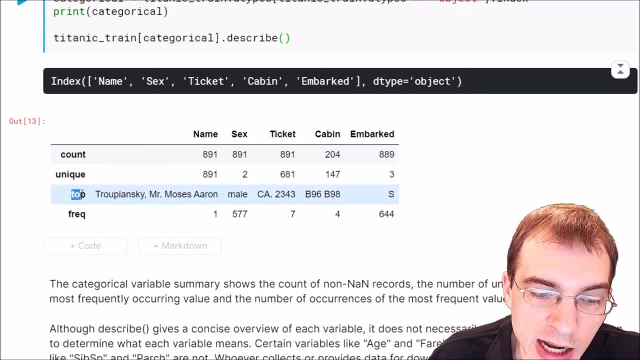 here. So that's probably male and female And then it's showing us top. the most common one is male And there were 577 male entries. So, as I alluded to earlier, when you load in a data set it's sometimes hard to make. 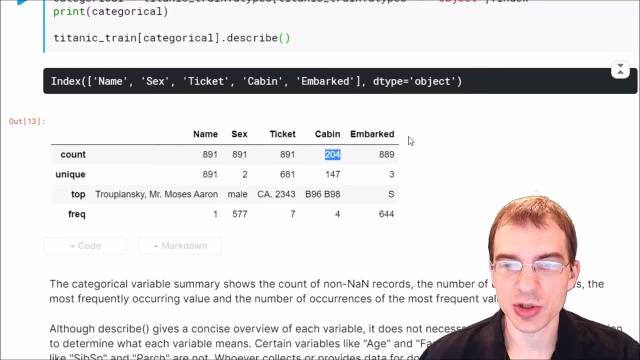 sense of the different columns without some sort of external explanation as to what the column is. So let's run this and see what the columns mean, especially if the column titles are not very explanatory of what's in the column. So with this competition and with many other Kaggle competitions and other data sets, you 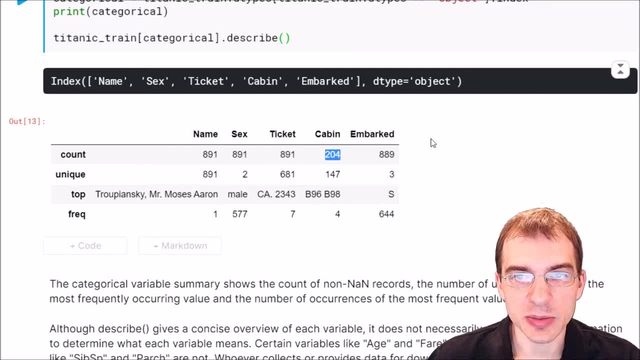 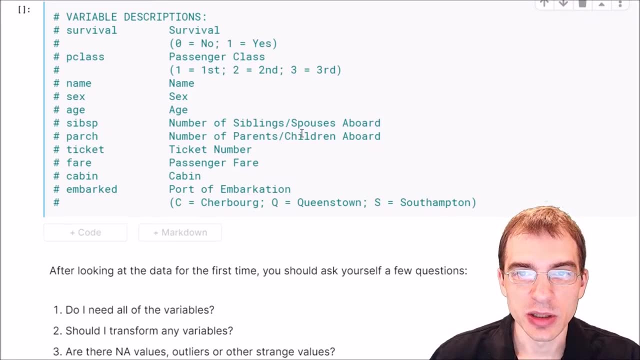 might find out there in the wild. you'll often have an accompanying document that provides some explanations as to what the columns actually mean. So this competition actually has that And I've included in here. So in this box it's just showing some explanations about what these variables mean. 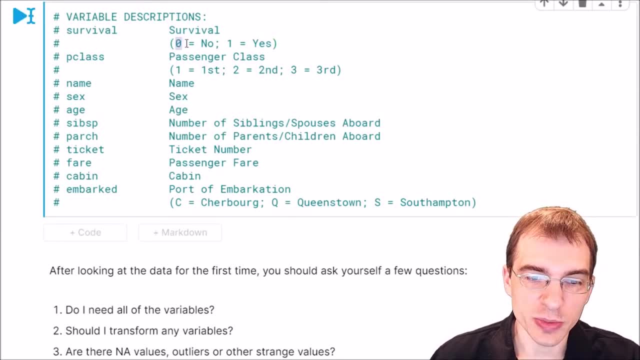 For instance, with the survive variable, a zero means no, the person didn't survive, And a one means yes, they did. So the importance of any kind of documentation like this for what the different variables in a data set mean cannot be understated, because having a good understanding of the variables 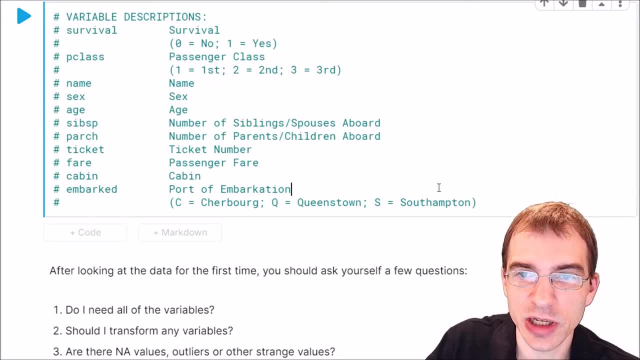 you're working with will be a great help in any sort of data analysis Or prediction task that you're doing. So after loading in data and doing some basic exploration for the first time, there are several questions you should be asking yourself to get the data ready for analysis. 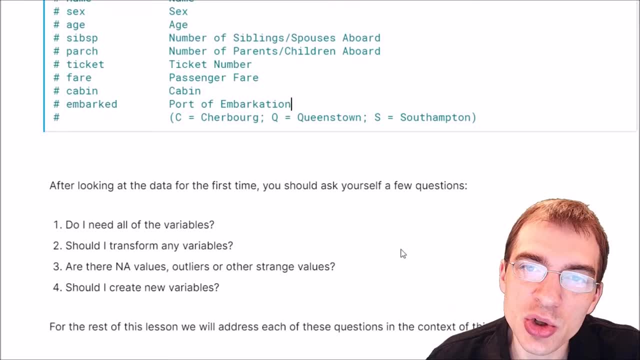 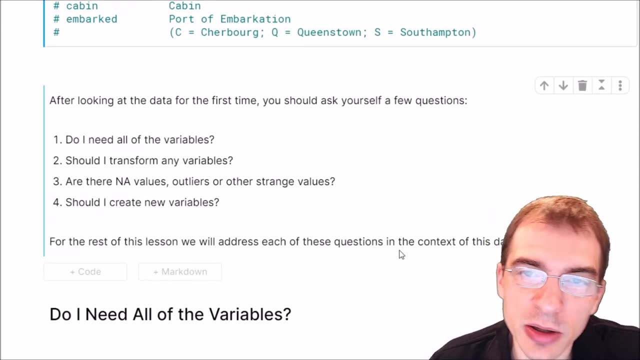 So we're going to list what some of those are and then go through each one in turn and look at different methods for achieving it. So one thing that you want to always be thinking about after loading in a new data set is: do you actually need all of the variables? 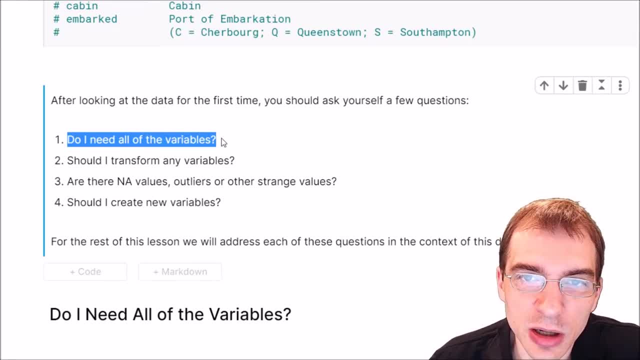 Oftentimes you'll have columns that either are just junk data that you don't want to use because they don't tell you anything, or they're data that aren't useful for whatever task you're trying to do, And by getting rid of it you might be able to free up some memory space and also, perhaps 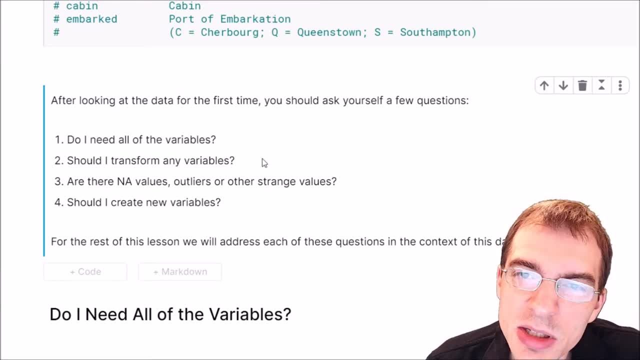 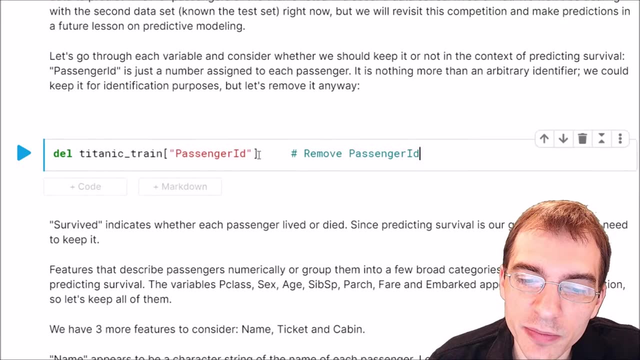 reduce unnecessary computation. So let's consider, with the Titanic disaster training data set that we loaded in, are there any variables we should think about getting rid of? Well, The idea of this particular data set is predicting whether passengers on the Titanic disaster survived or not. 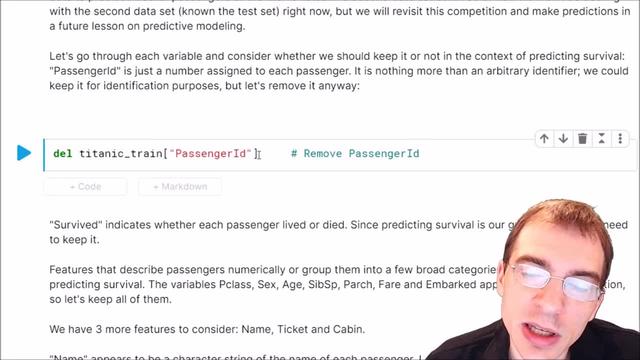 So in terms of that end goal, we can kind of already see there's probably one variable that we could remove, the passenger ID variable, Because when we were looking at the description of that variable it was simply just a counter that was counting each of the rows one through 891.. 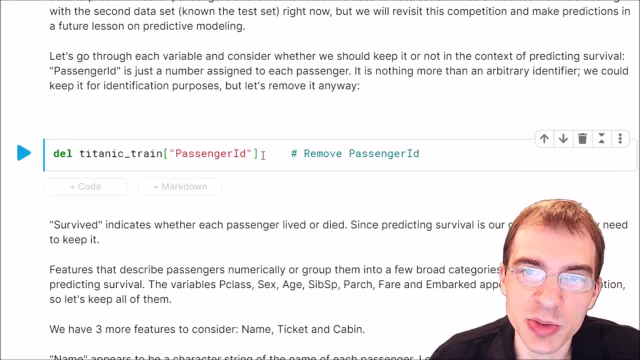 So the passenger ID is just an arbitrary variable. It's an arbitrary number that's been assigned to these different records and really has nothing to do with whether that person was going to survive or not. So for this task we could safely remove that variable and probably would actually want. 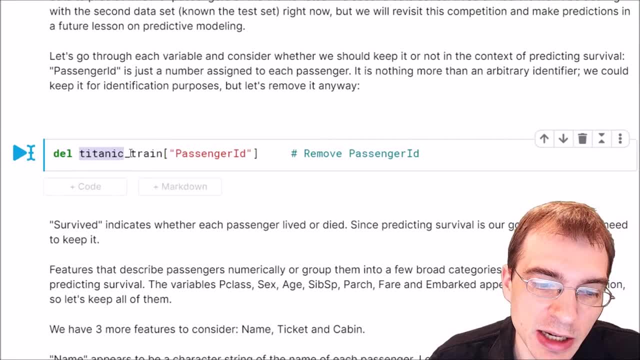 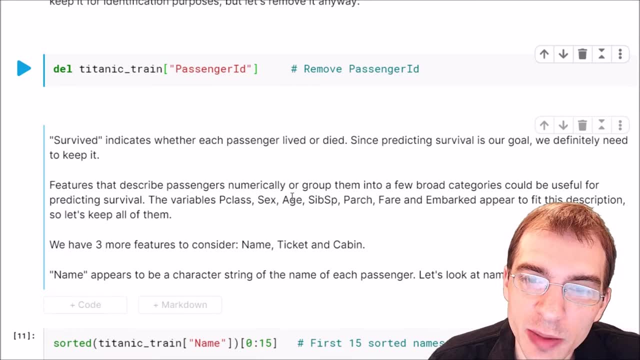 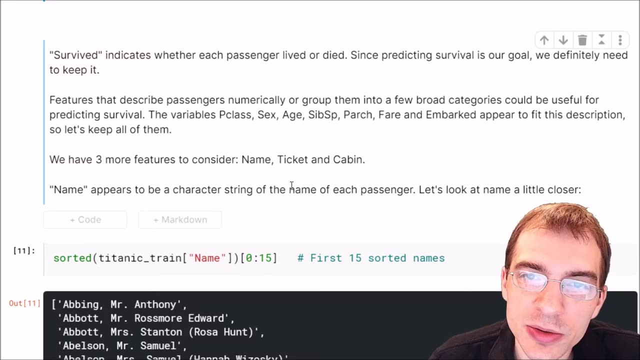 to remove it. So let's start off by saying: delete Titanic train passenger ID. Now the numeric columns that we looked at, as well as the categorical ones that describe passengers in broad categories such as sex and class and age, Those are things that would probably be somewhat useful for prediction. 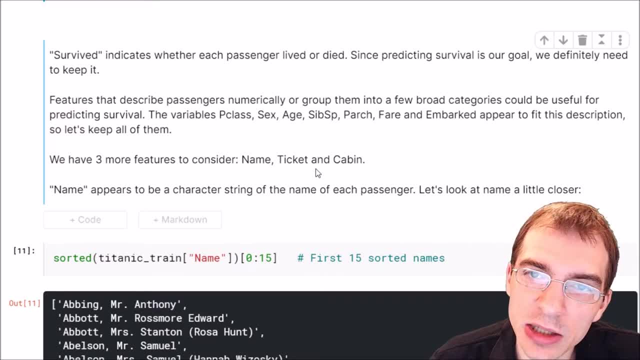 So I would say we should keep those. but we have a few other categorical variables that might be somewhat questionable as to whether they're going to be useful for prediction or not. Those would be the name variable, ticket and cabin, Because when we looked at those they had a lot of different unique values and it was 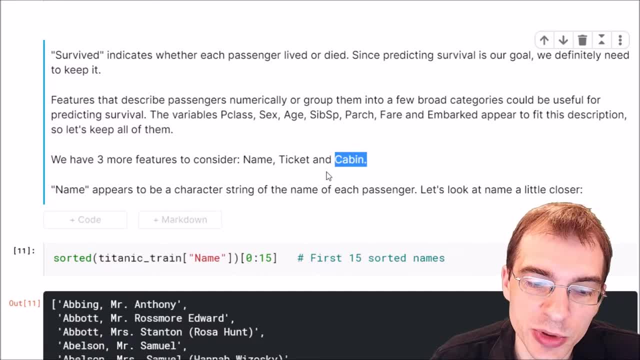 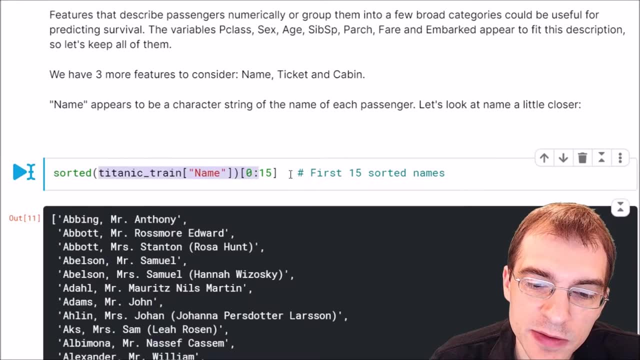 unclear whether that would be something that would be useful for doing prediction. So let's start by looking at the name variable a little closer. We're going to sort it And then just look at the first 15 sorted names. So let's scroll down here and we see it's just a bunch of full names for passengers. 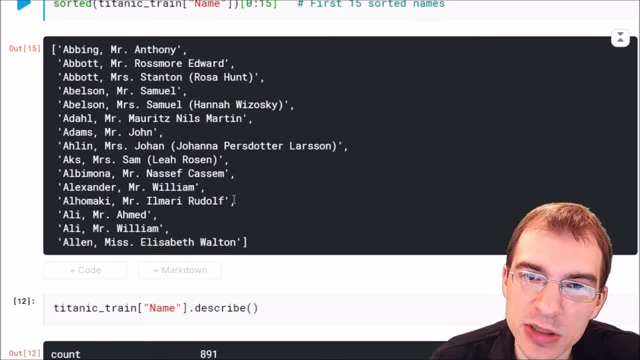 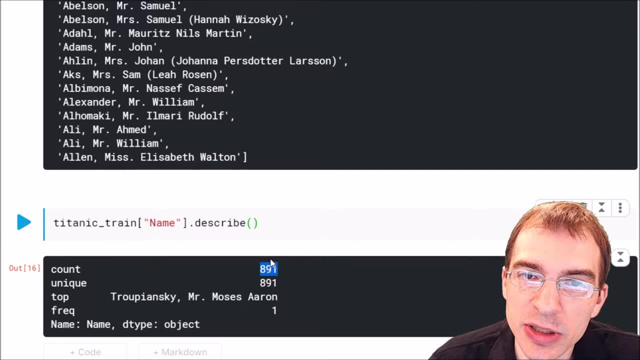 And what really does a person's name tell you about whether they're going to survive or not? In fact, if we run describe on the name variable, we see that there are 891 unique names. That's not really a surprise. Every person has their own unique name. 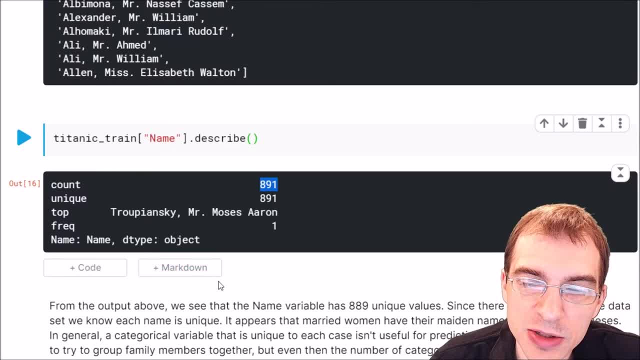 So, unless we wanted to try to run some sort of text processing steps on these actual names, this is a variable, So let's try to run some sort of text processing steps on these actual names And we'll see that this is a very good way to run the text processing. 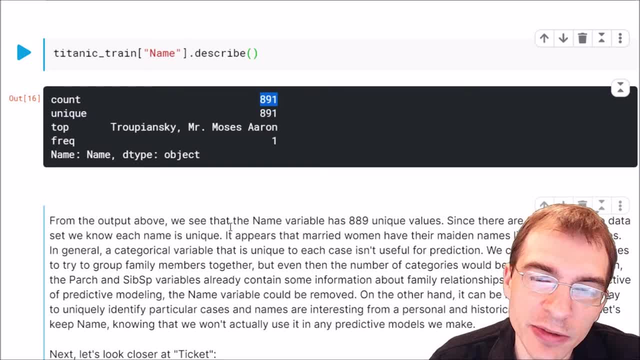 For example, if I had a number that said passenger ID and passenger ID, I'd probably remove for this prediction task. But in this case it'd be nice to have some unique identifier for each of the records And we already removed the passenger ID unique identifier. 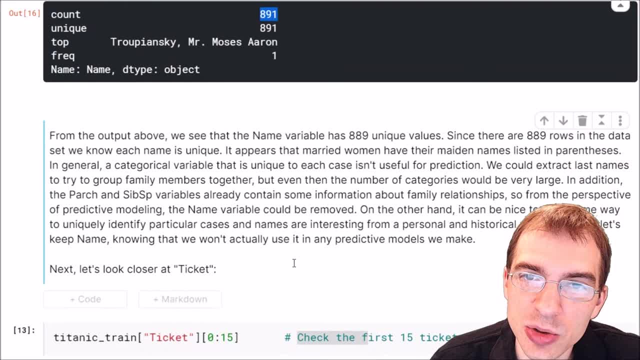 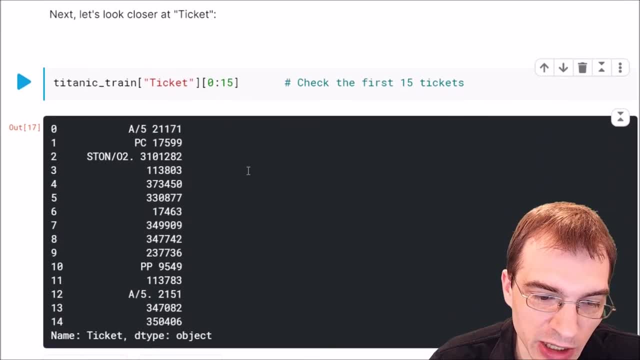 So for now we'll just keep this, but it's not something we'd probably want to use to be predicting with. Next, let's go ahead and look at the ticket variable. So we'll look at the first 15 entries of that And we can see here the tickets really don't seem to have any rhyme or reason for their. 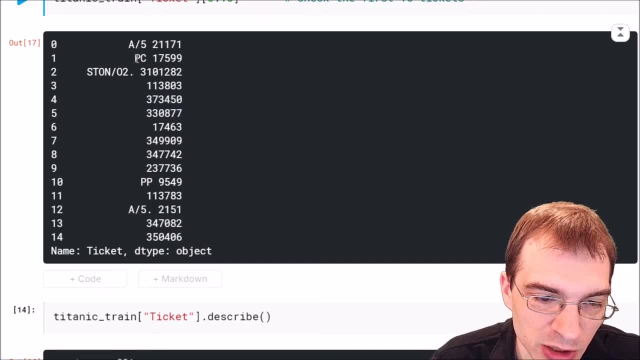 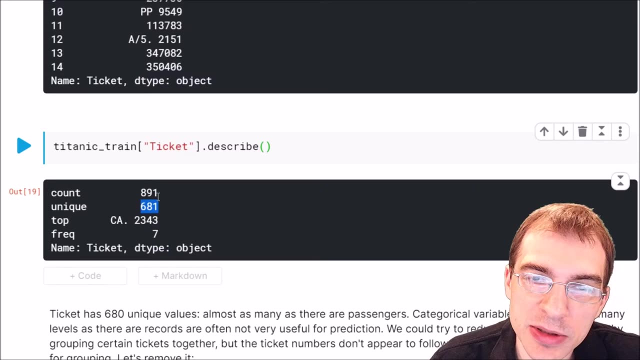 structure that are just pure numbers. we have ones that are a mixture of letters and numbers, even like a slash in that one. let's also run dot describe on it to see how many different unique entries and whatnot we have, and we can see there are actually 681 unique cabins listed. so when a categorical 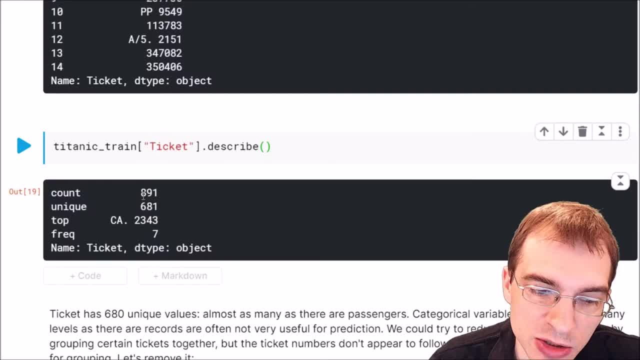 variable has almost as many unique values as there are total records. it's usually suspect, as, in terms of whether it will be useful for prediction or not, we could try to reduce the number of different levels by somehow combining things into different groups, but i think in this case it's messy enough. 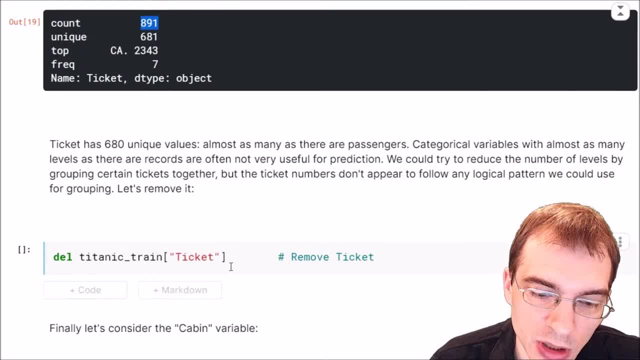 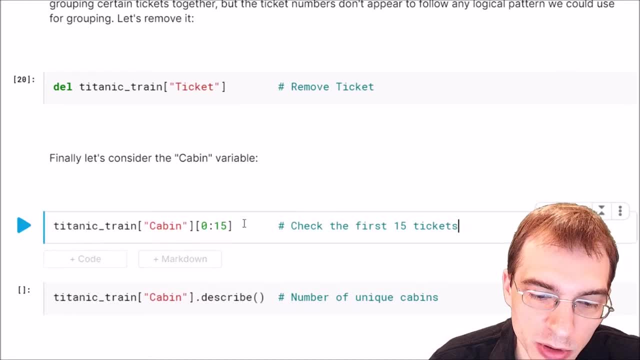 and there's enough unique values in it that i don't think we're going to use it. so let's go ahead and delete the ticket column as well now, finally, let's look at that cabin column. we're going to pull up the first 15 rows for that, and when we look at that, we see: 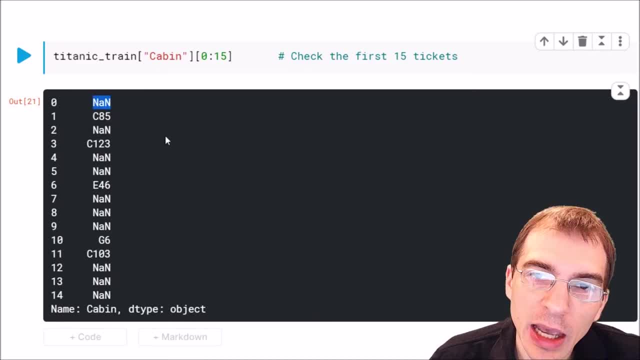 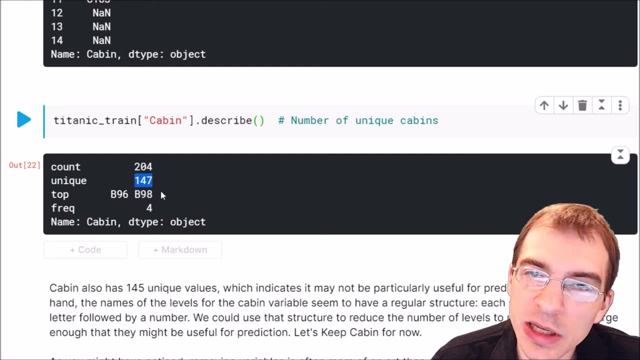 there are quite a few missing or not a number values and if we run describe on it, we see that there are fewer unique values. this time there are only 147 unique values, but there are also only 204 counted values, because most of them are missing, since most of the 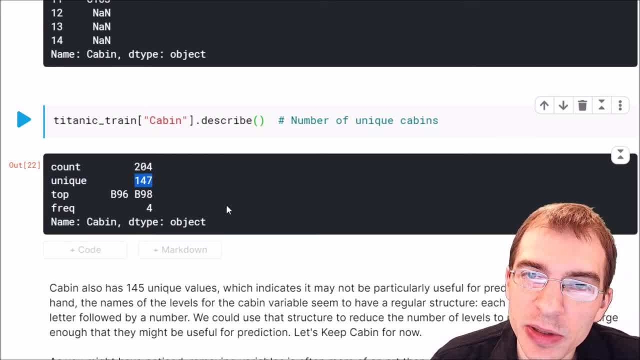 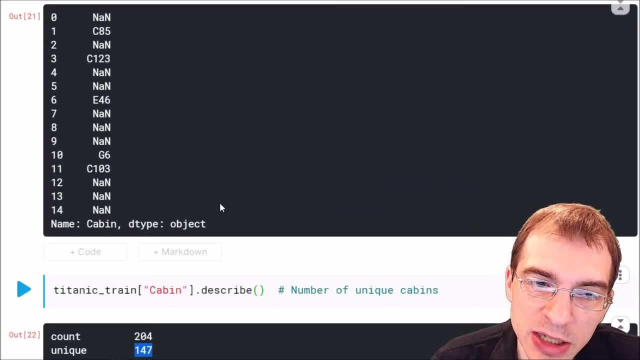 non-missing cabin values are unique. we could probably think that this isn't going to be useful for prediction, but we can also notice above that the cabins have a letter designation on them that is common across a lot of different numerical cabin numbers. so here we see c85, c123, c103. so in this case this letter designation c could be a way of grouping. 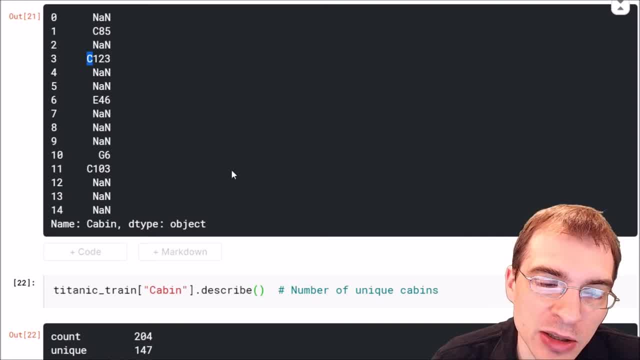 categories together in a way that might actually be logical. say, there might be a section c on the ship where all of these different c numbered cabins are in that area and it could be that a certain designated section like that in the ship, people were more likely to die in that area. 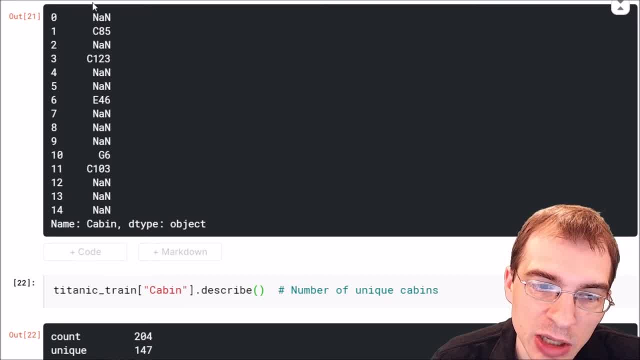 depending on how the crash happened and where the section was located. so this variable still might actually have some value for us in prediction if we can extract that information into some meaningful groups. so we will leave the cabin variable here for now and see if we can deal. 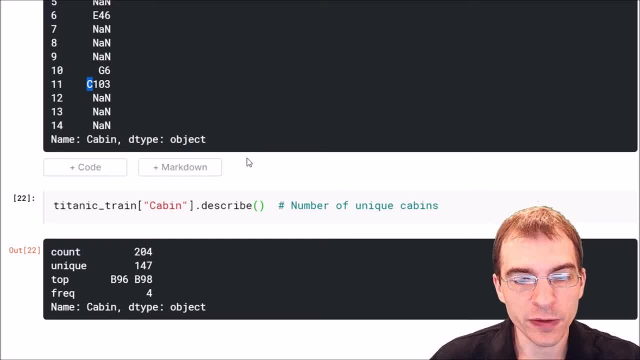 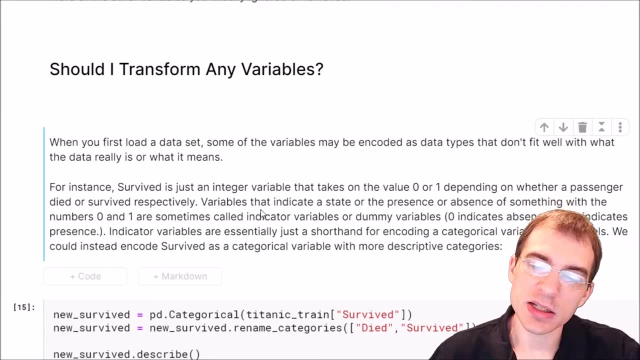 with that later. so now that we've considered whether we should remove variables, we should also be considering should you transform any variables. for instance, when you first load a data set, some of your variables might be encoded as data types that don't fit particularly well with what you're trying to do. for instance, if your data had, say, dates and they were loaded. 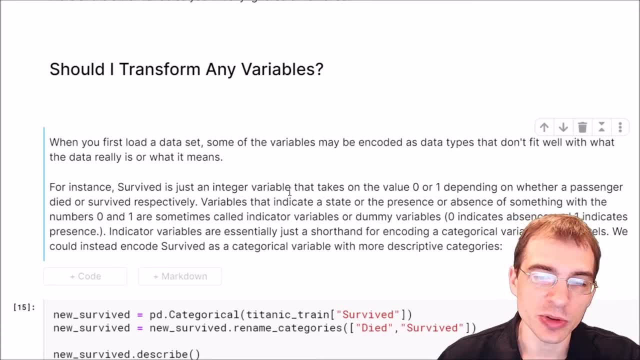 in as strings or numbers and you wanted them as dates. well, you might have to convert them to actual date objects. in our data set, the survive variable was loaded in as zeros or ones, depending on whether they survived or died. but if that's not such a nice way of thinking, 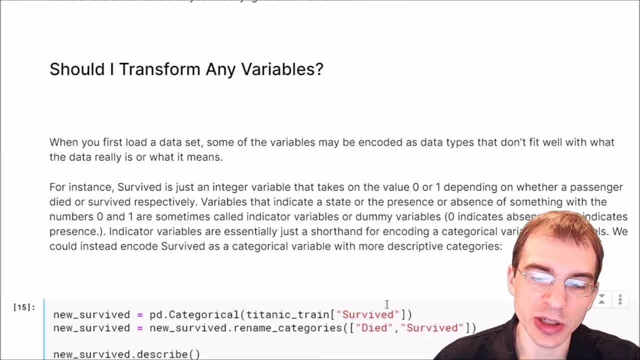 about it. it'd probably be easier to think about if we just had the full string- died or survived, so we don't have to think about it in terms of zeros and ones. so as a simple example of a transformation, we could turn the survive column into categorical to cast something as a categorical. 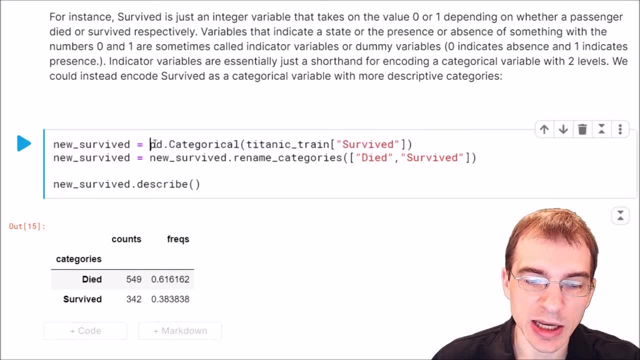 variable. we can use the pandas function pdcategorical- and then we will pass in the column survive that we want to transform. so after we do that and save it as a new variable, we'll also run this operation on it to change the names of the categories. so we're going to take our 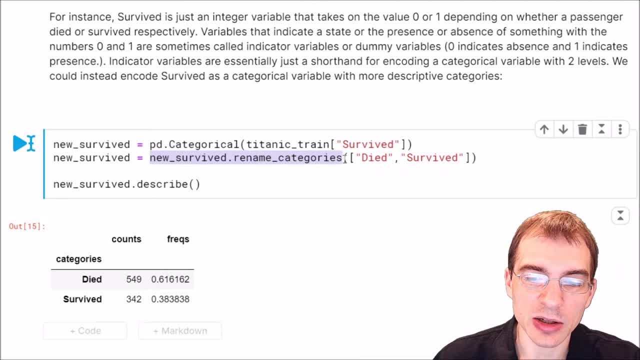 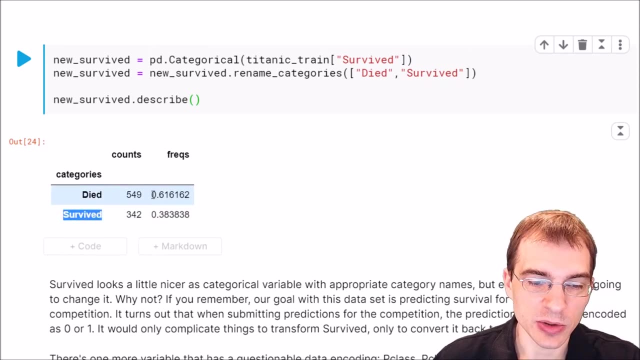 new survived data and dot rename the categories to these died and survived. after we do that, we can run dot describe on our new variable, just to look at a table of it now. so now we have some nice categories that are easy to understand and we can see the frequencies here where 61 percent of people died and 38 ish percent survived. we also 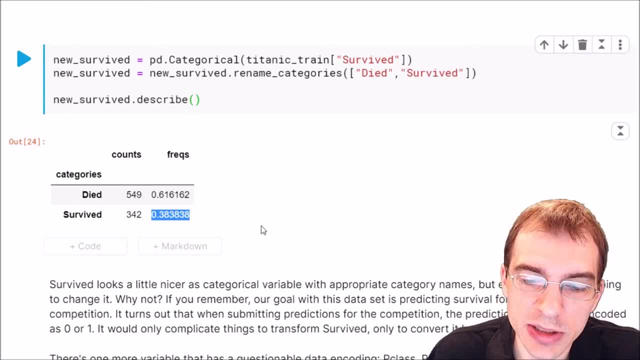 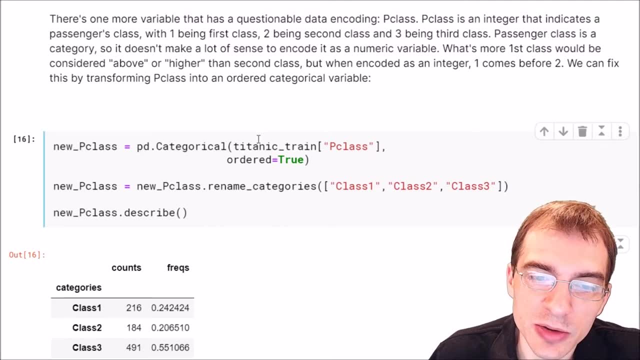 noticed another variable earlier that actually has questionable data encoding, and that is the p class or class variable. the p class can has three different values: 1 for being first class, 2 for being second class and 3 for being third class. This variable was loaded in as an integer number. 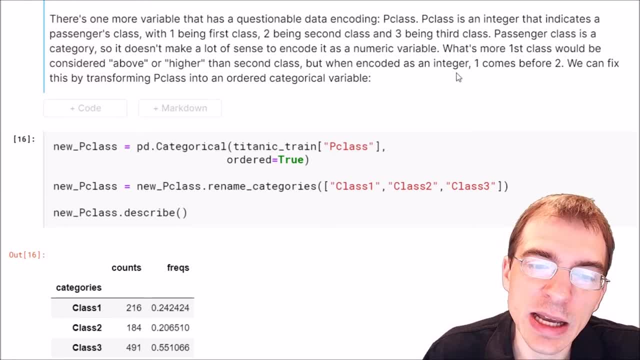 even though we know intuitively that passenger classes are actually categories. So it doesn't make a lot of sense to encode that as a numeric or integer variable. What's more, first class would be considered to be above or higher than second class, but first class was encoded as the integer 1, which is actually before or lower than 2.. 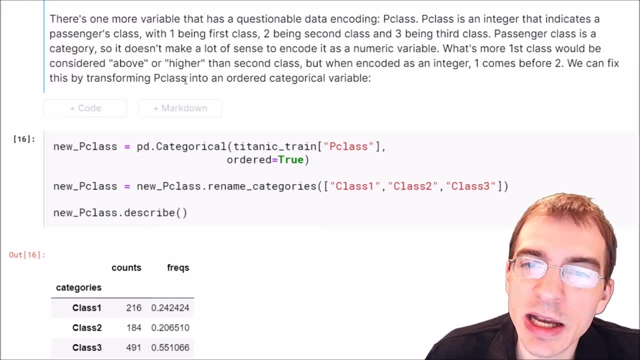 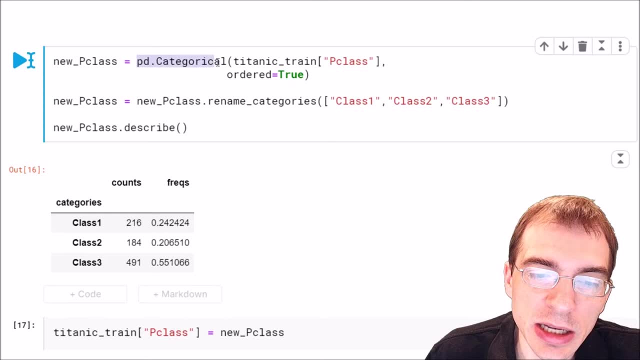 So we could address this by transforming the pclass variable into an ordered categorical variable. So we'll show how to do that here. Again, we can run pdcategorical on our pclass column and to make it an ordered categorical variable, we can add this additional argument. 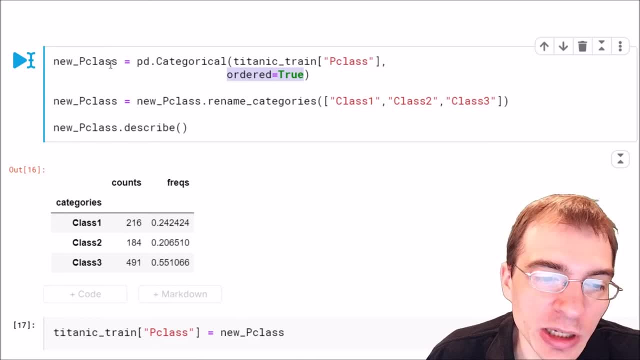 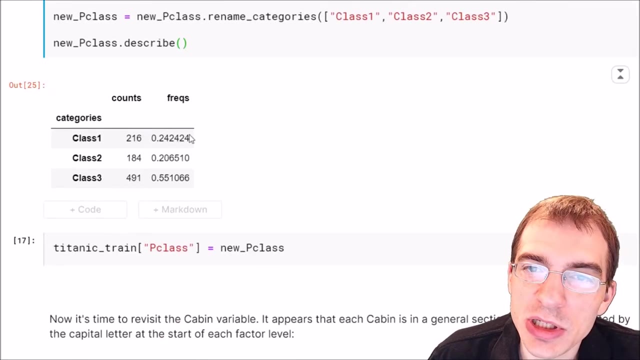 so comma ordered equals true, And after creating this new pclass variable, that's categorical- we'll just do rename categories again, so we can give them names that we can easily understand: Class 1,, Class 2,, Class 3.. And now, instead of a numerical summary, that perhaps wasn't particularly useful before. 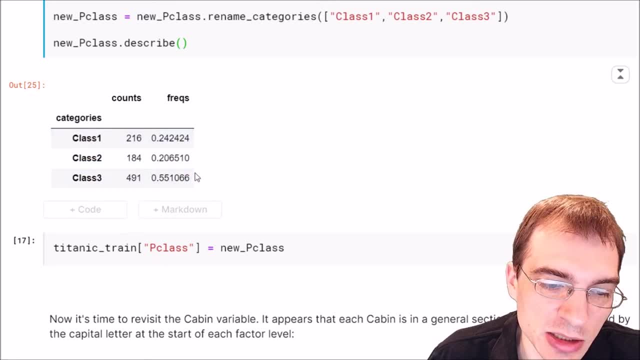 we get a summary of the categorical version of pclass and this gives us a bit more interesting information. here We can see that about 25% of the passengers here were in first class, 20% were in second class and 55% were in third class. 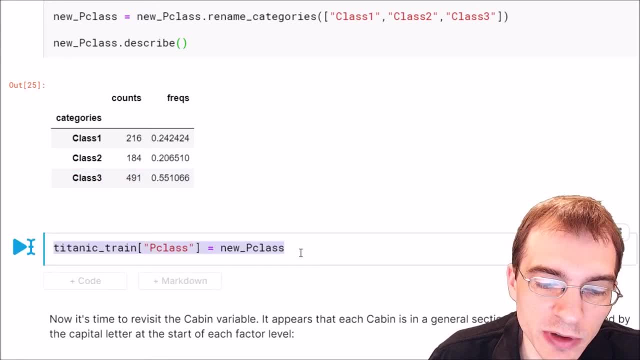 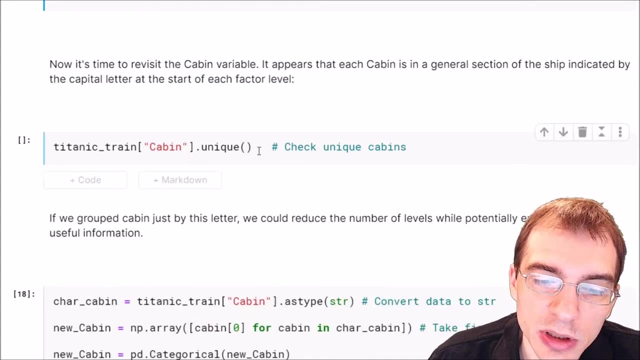 So let's go ahead and overwrite our original pclass variable with this new categorical version. And now it's time to revisit our cabin variable that we didn't remove before. If we run unique on cabin, we can see that it has a bunch of unique values. 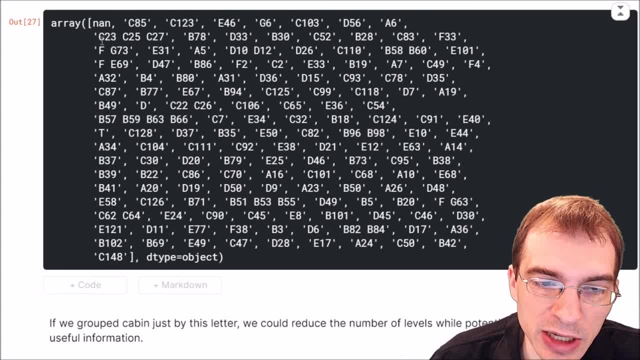 but again, many of them start with the same letter designation. We have like C, E, B, A. So let's group the cabins by the letter designation and hopefully we can reduce the number of unique categories and perhaps extend them. 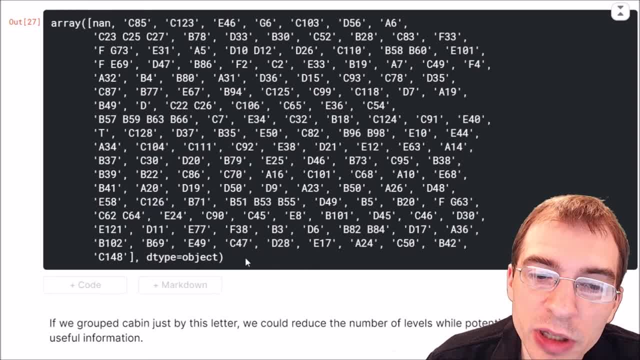 So let's go ahead and extract something useful from this variable. So what we want to do here is just extract the first letter of each of these cabin strings and then create a new categorical variable that's just based on that letter instead of the numerical portion. 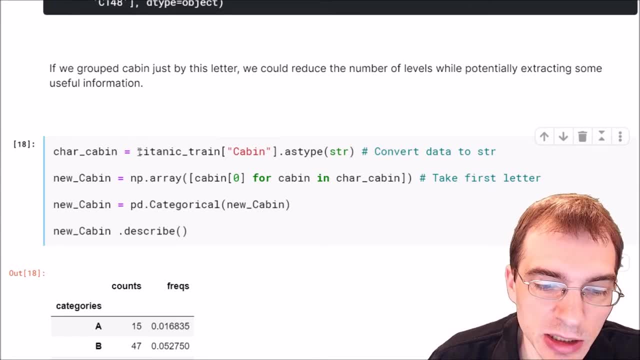 So we'll show how we could do that below. We're going to start by getting the cabin variable. That's what this is doing. Then we're going to first encode it as type string, because when we loaded everything in, they were encoded as object types. 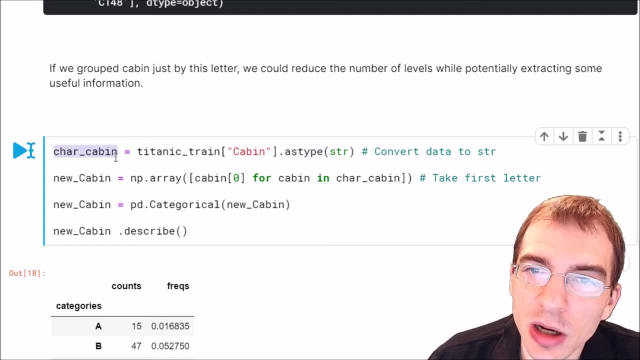 Now we're going to run a list of things that we're going to need to do. So we're going to do a list comprehension on this column to extract the first letter from each record. So this is the list comprehension we're going to run here. 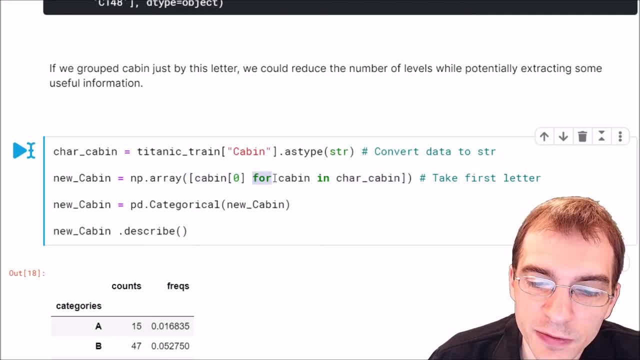 Cabin zero. that's saying, get the first letter for each cabin in the cabin variable that we just saved. So this list comprehension is stripping off the first letter of every single record of the variable And then we're just wrapping this whole thing in nparray. 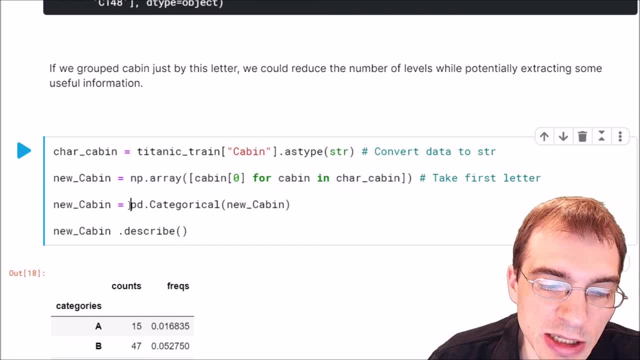 to turn this into a numpy array. We're running pdcategorical on the array to transform it into a new categorical variable And now we'll run describe on that new variable to check what we got here So we can see after running this. 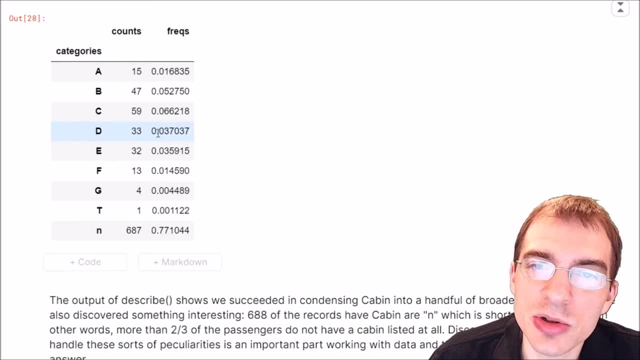 we have managed to condense that cabin variable down into much fewer categories. So although many of the variables were missing here, these are the missing ones- 77% didn't have a cabin listed. We have far fewer unique categories, So some of these might actually be useful for prediction. 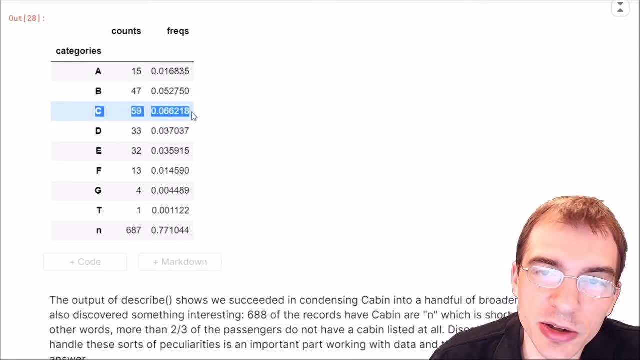 For instance, there are almost 60 people In the C area of the ship, 47 people in the B area and quite a number in the D and E areas. So potentially that could be useful for prediction, For instance if area D was the spot on the ship where the crash occurred. 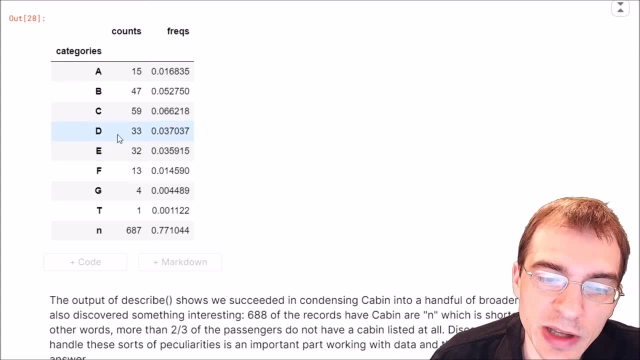 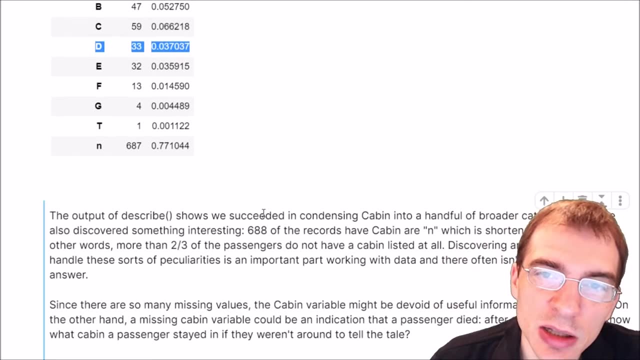 perhaps everyone in that whole section didn't survive, And if that was the case, this D variable could be a powerful predictor for not surviving. Since this could potentially be useful, let's go ahead and save over the original cabin variable with our new cabin variable. 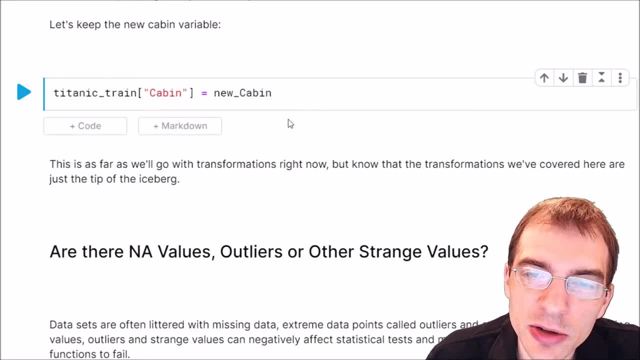 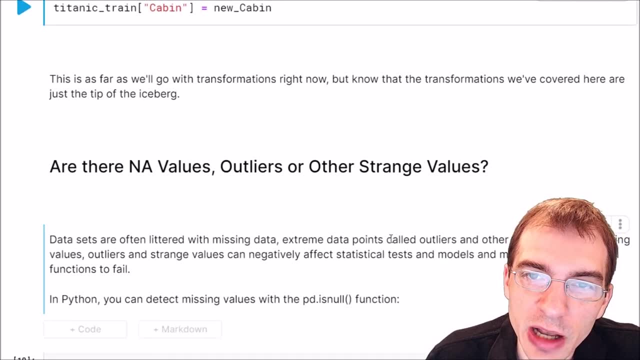 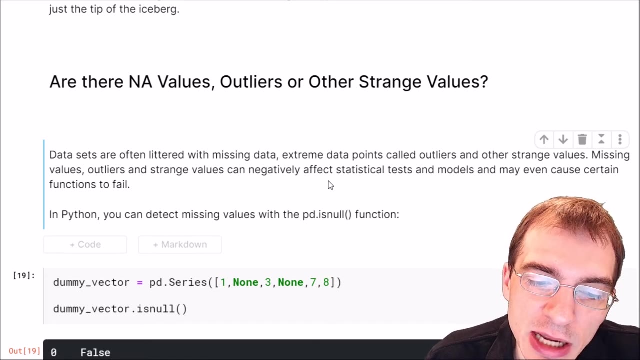 Now that we've done some variable transformations, another question that we should consider is: are there any NA or missing values, outliers or other strange values we should deal with before proceeding with any kind of analysis? In Python, using the pandas library, you can detect whether there are any missing values with pdisnull. 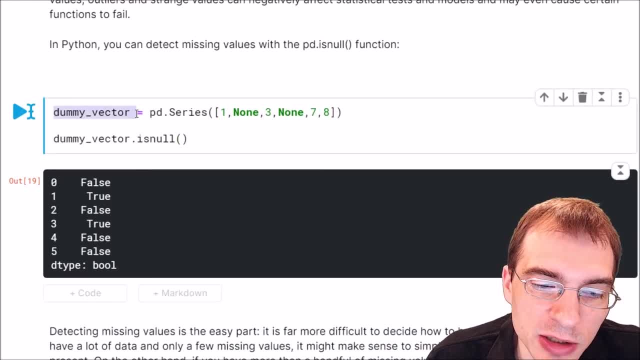 So we'll just give an example of doing that. We'll create a dummy vector of data that has some none or missing values and then we'll run dot is null on this dummy vector and it'll just produce logical output where, if the value is, 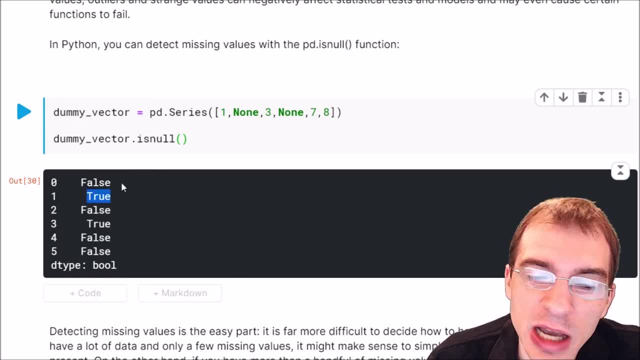 missing or null, a true will be listed and if it is not, a false will be listed. So we can see, in this case in exposition, one and three were true because we put missing or none values in for those. So identifying missing values is the easy part. 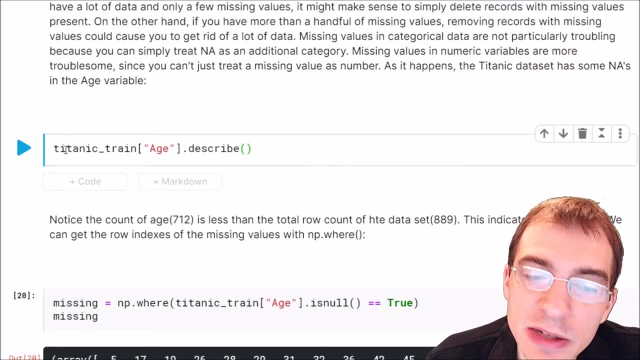 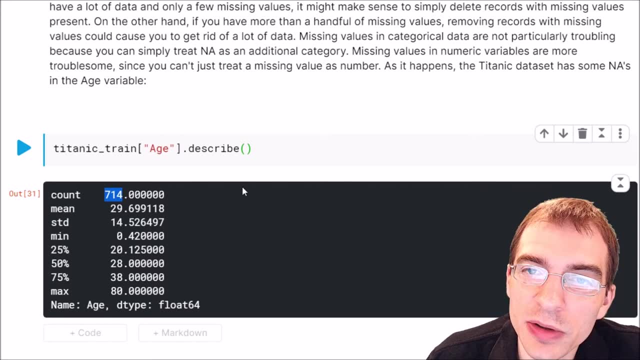 It's much harder to decide exactly how to handle them. For instance, if we check the age table in the Titanic data and run dot describe on it, we see that the count here is actually fewer than the total number of records. So let's identify the indices where these missing age values occur. 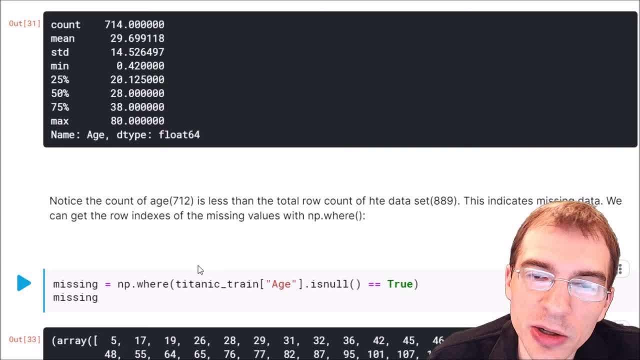 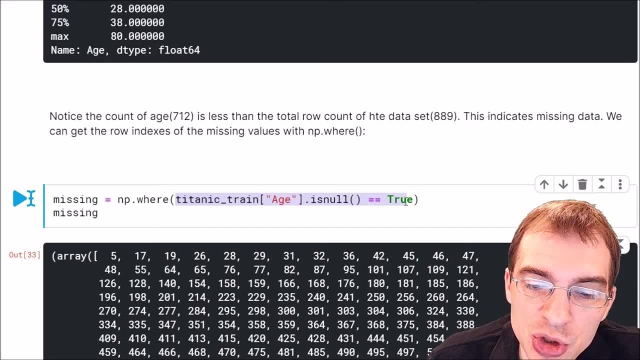 We can use the is null construction that we made earlier to do this, so we can use the same construction above Titanic. train age is null And we want to check where that is true And we're going to use this whole thing within an npwhere clause. 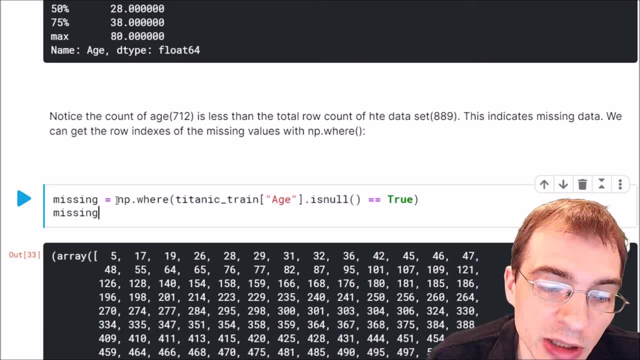 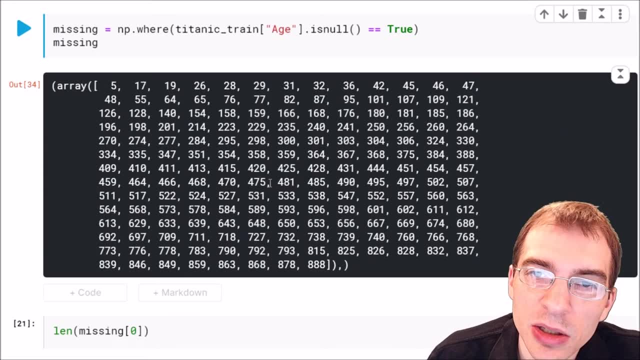 It will extract the corresponding indices. So by running this we're going to get all of the indices where the value is missing. So here we have an array of indices where the corresponding age value is missing, And this is quite a few missing values. 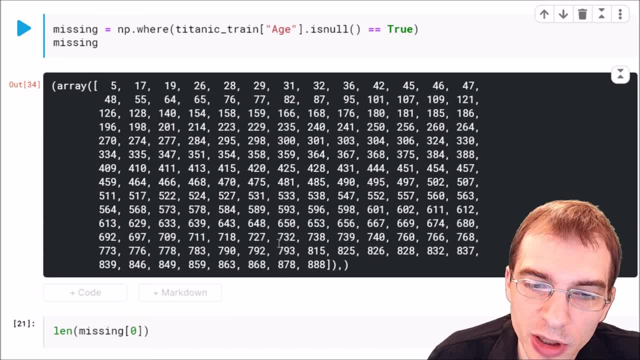 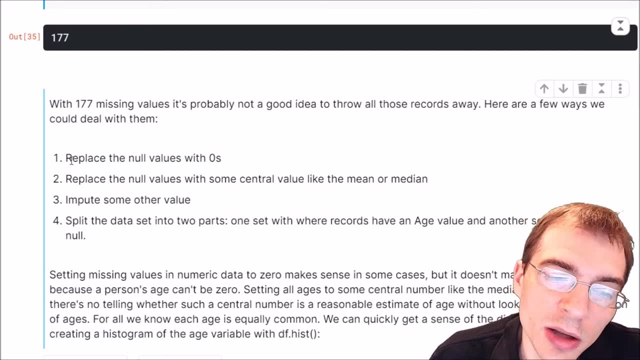 So we definitely need to do something with this before we continue with our prediction task. So when you see missing values in a data set, there are a number of different things you could consider doing to them. One: you could replace all the null values. 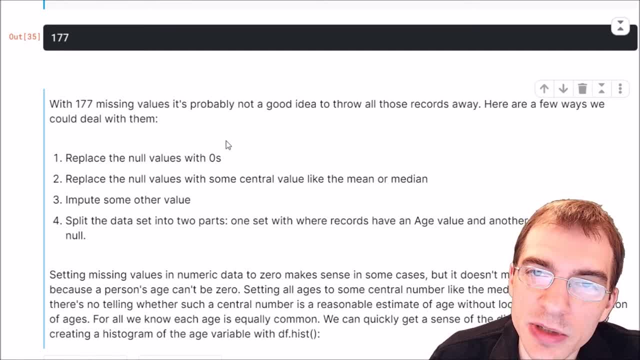 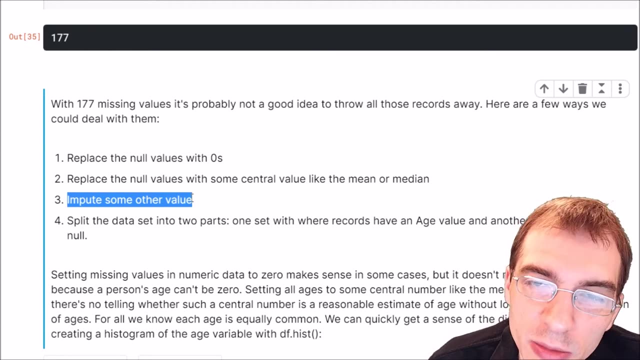 with zeros, if you happen to be working with numeric data. anyway, You could replace all of the missing values with some central value like the mean or median of the column. You could try to impute some other value. Imputation means using some sort of algorithm to fill in the values. 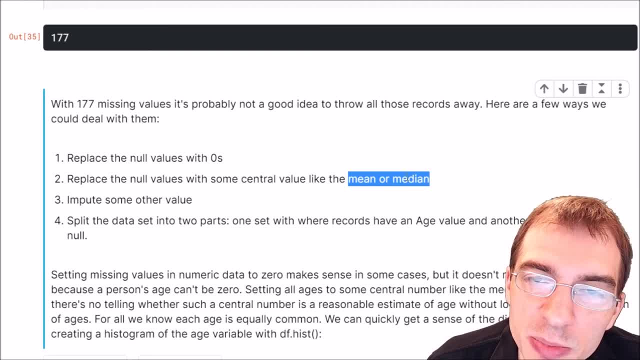 In fact, mean and median are simple forms of imputation, But there are other, more complicated forms of imputation, say using data in other columns to try to make a guess at what would be reasonable values for the age column. Another possibility would be splitting the data set into two parts. 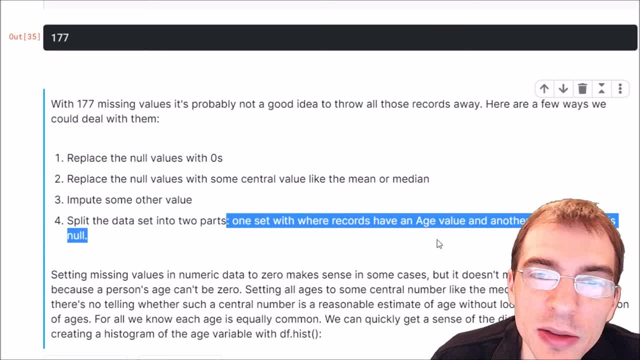 one where the age variable is not missing and the other where it is missing. Now, setting all of the missing ages to some central number like the median or mean age could be a reasonable thing to do, except we don't know exactly what the distribution. 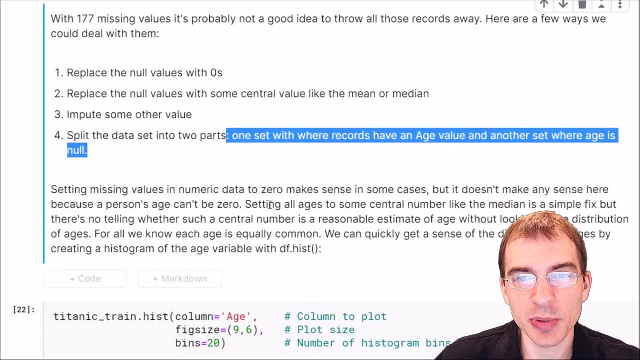 of the age variable looks like yet. So to do that, we could pull up a quick histogram of the age variable to see if it looks like a fairly normally distributed variable And if it is perhaps using the mean or median would be a reasonable thing to do. 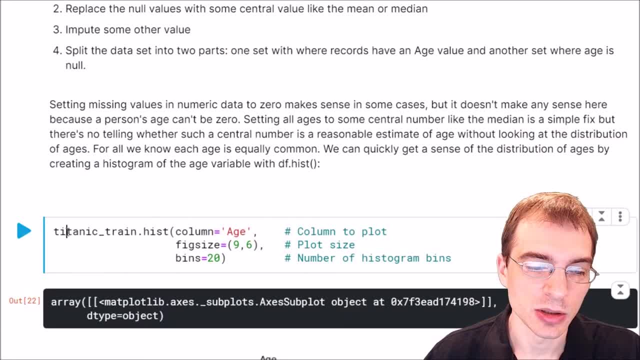 So we'll show how to make a simple histogram. in pandas You pass the name of the data frame, dot, hist, And then within this you say: column equals whatever column you want to plot, And these are just specifying the size of the figure and the number of bins we want in the histogram. 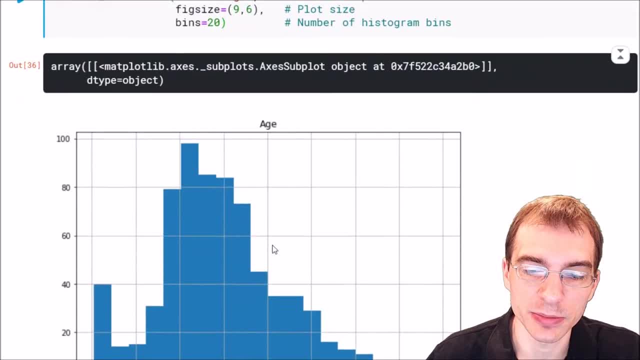 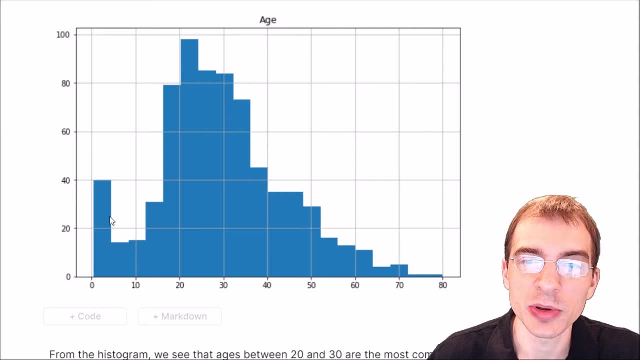 When we run this, we should create a histogram of the age column So we can see that while there is some concentration of ages at the low end, so there were some younger people on the ship. In general, the data seems to follow a somewhat normal pattern here. 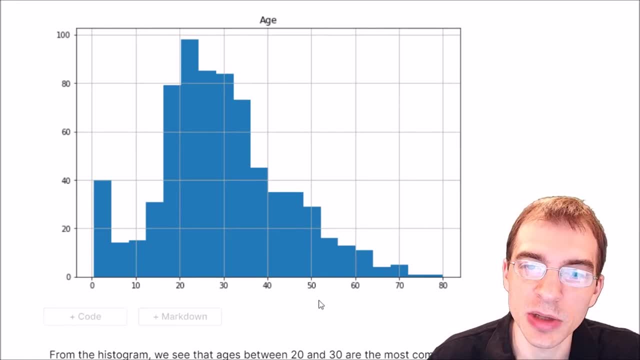 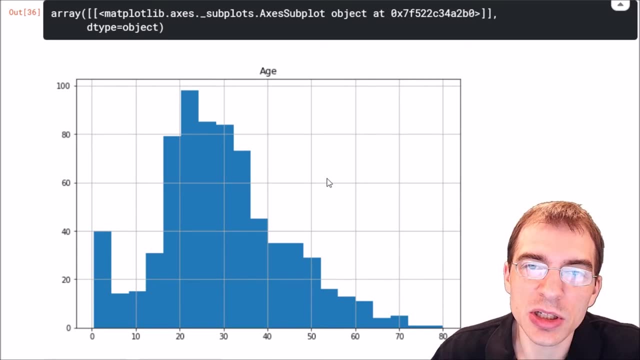 So perhaps setting the missing values to some middle value age between, say, 25 or 30, might be a reasonable thing to do. So let's go ahead and set the missing age values to the median value of 28.. And we'll show how to do that below. 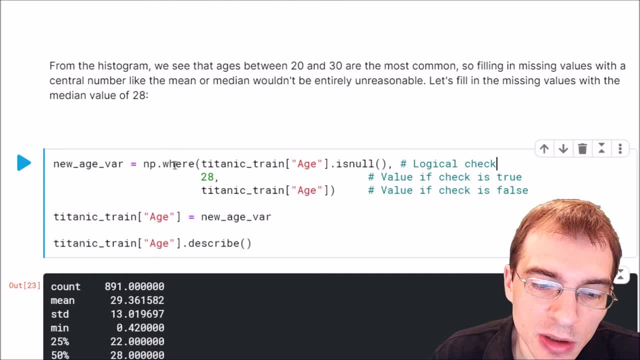 So we can use the NP dot where function to do this. We will say NP dot where. then a logical check. In this case, we want to check where Titanic train age is null And when this is true, we're going to set the value to 28.. 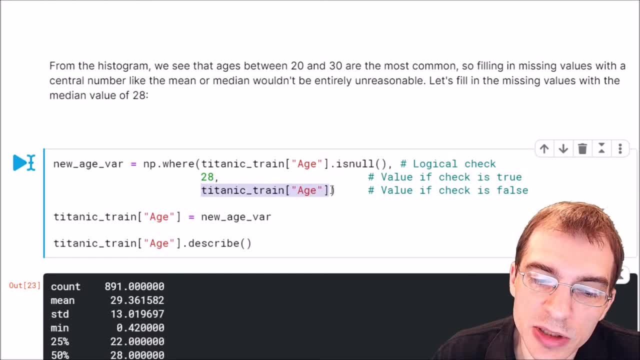 And where this is false, we're just going to keep the original value. that's actually there and that will give us our new age variable And we'll just overwrite the original age variable with our new one And then we'll run dot describe on it. 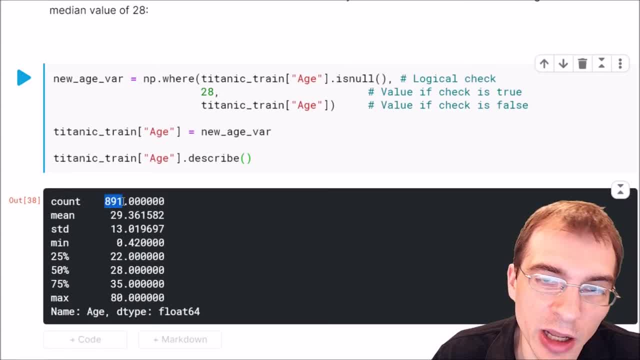 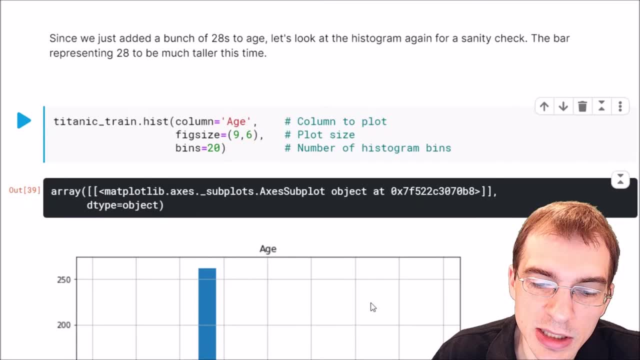 to just confirm that we do indeed have a count of 891 now, So all of those missing values were overwritten. Let's go ahead and rerun our histogram as well, Just to get a sense of what the data look like. now You can see that by assigning all the missing values, the value of 28,. 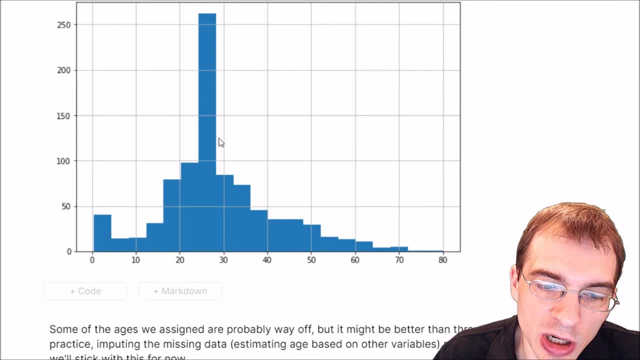 this bin, where 28 lies, is much taller now because there's a whole bunch of extra values in there. Now, clearly, some of these age values we imputed with the median are going to be quite a bit off from their actual values. On the other hand, doing this might be better than throwing entire records away. 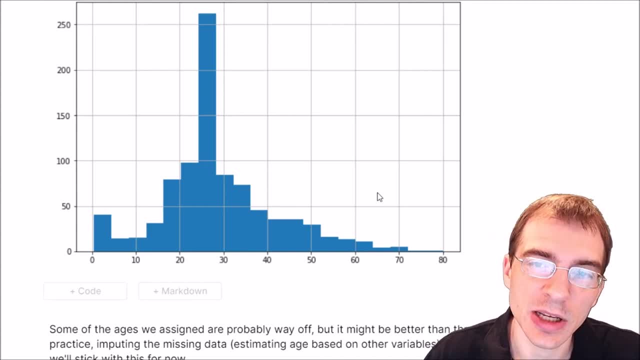 These are the sorts of decisions you'll have to be making in data analysis projects oftentimes- And there's often really no one right answer as to what the best thing to do is. It often is just a matter of having experience and knowing a lot about the domain that you're working in. 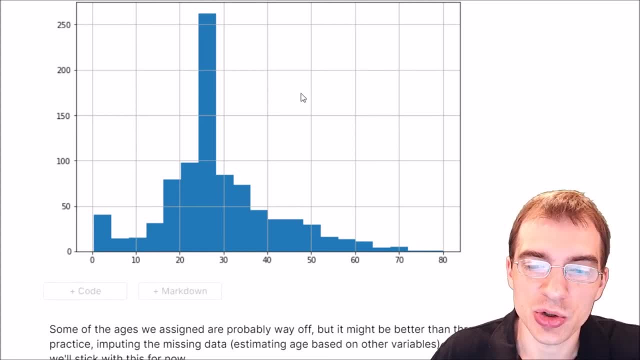 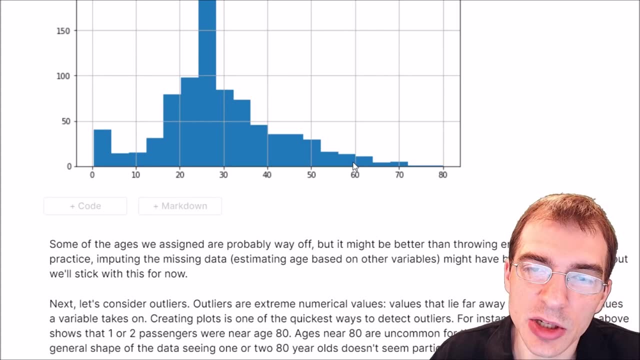 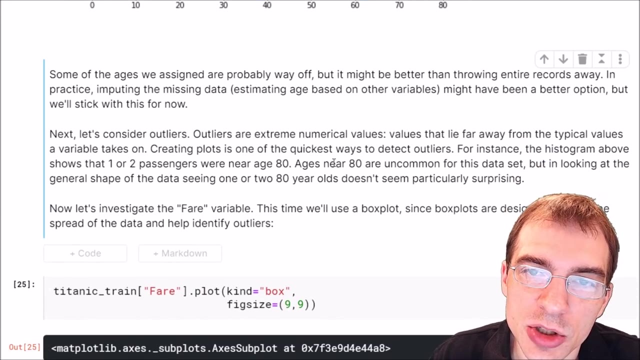 Now let's consider outliers. Outliers are extreme values that lie far away from the typical values within a distribution. If a data set has some extreme outliers, they can have significant negative impact on various predictive modeling techniques. So it's good to identify them and perhaps do something to them to deal with that. 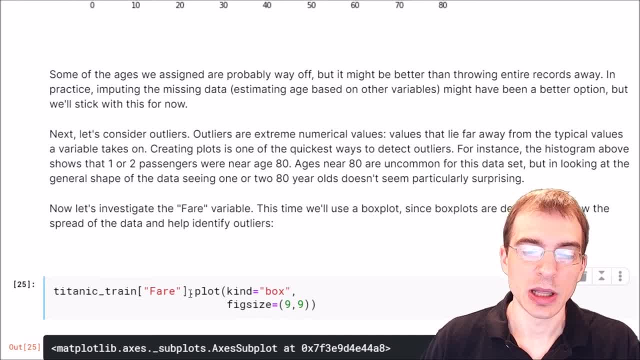 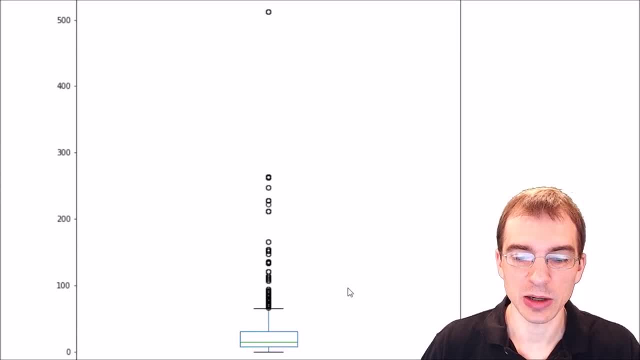 To look at some outliers. let's check the fair variable. I'm going to run dot plot, kind box on it to make a box plot And this sort of plot is good for detecting outliers. Here we see on the box plot, this green line is the median value. 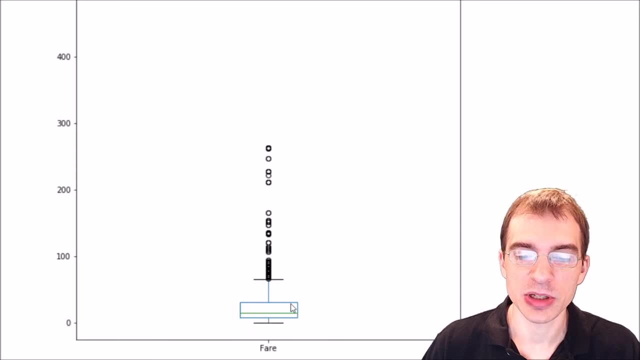 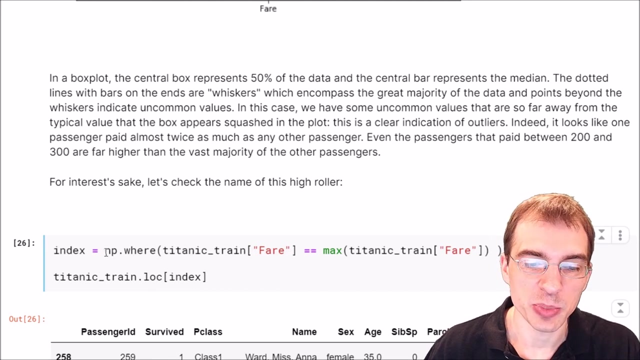 And this blue box contains the middle 50 percent of values. So some of these circles above the box are way above the median. Out of interest, let's determine who actually was this person or people that paid so much for their tickets. So to do that, we can run NP dot where on the fair column, where the fair is equal. 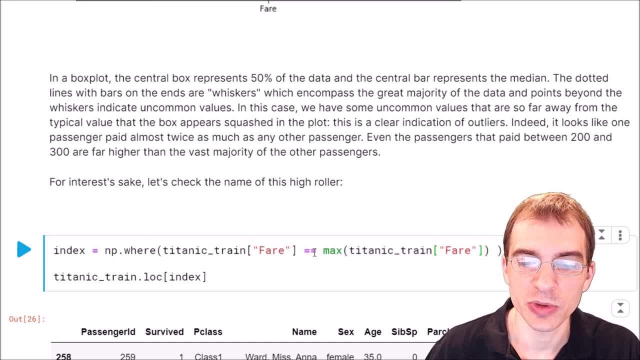 to the max of that column because we want to see who the biggest one was. So that should be the max. And if we do that, save that index and use it to index into the data set. We can find who that person is, so we can see. 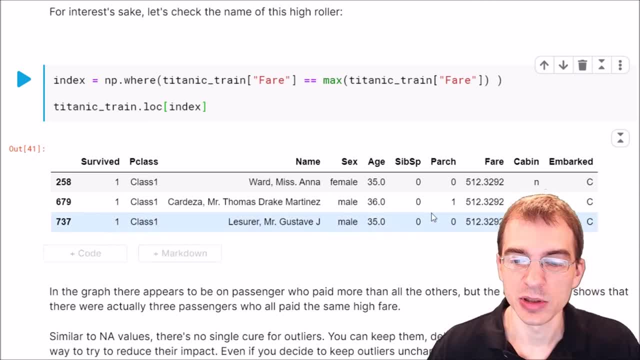 There's actually three people that all paid the same amount. They paid five hundred and twelve, either dollars or pounds or whatever the fair value is, and all of these people were in first class. Well, you should hope that they would be if they paid so much. 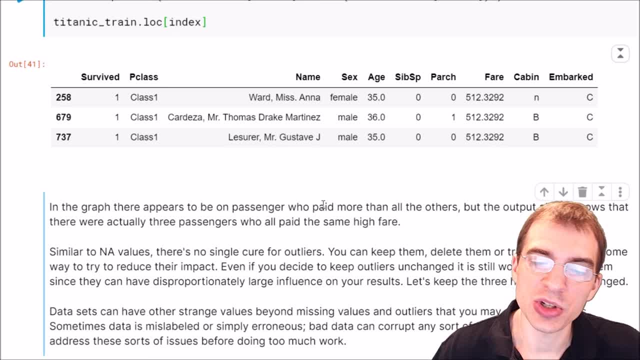 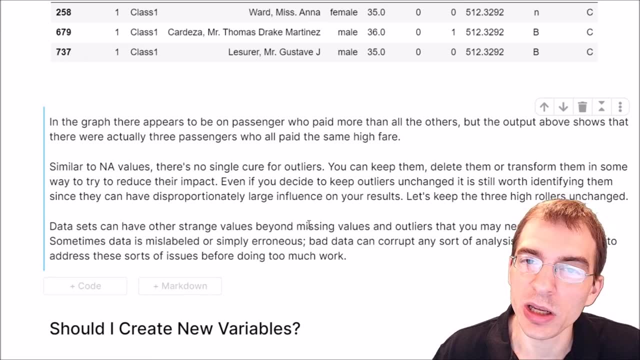 Now similar to any or missing values. there's no single cure for what to do with outliers. We could keep them in, We could delete them, We could try to transform them in some way to reduce their impact or select modeling techniques that are not bad. 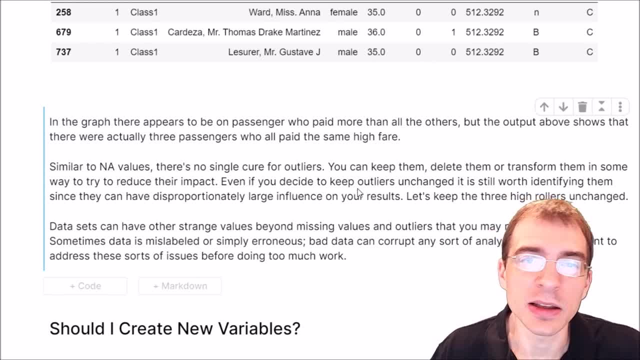 It's not necessarily completely affected by outliers, but it's still worth identifying them and keeping them in the back of your mind, because they can't have a disproportionately large influence on your results. So we're going to keep these high rollers in our data set. 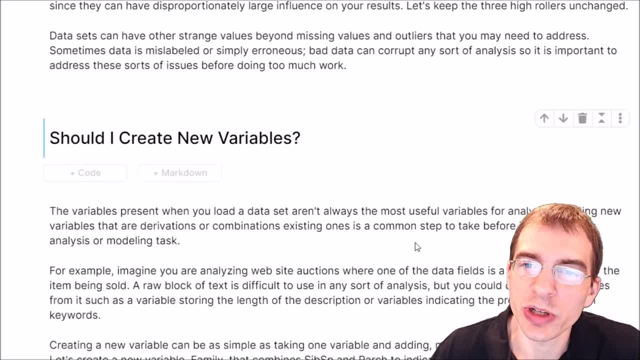 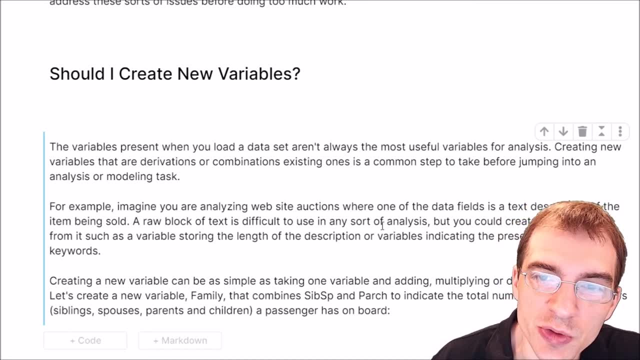 But it's a good thing we know that they're there. One final thing to consider is: should we create any new variables? So when you first load in a data set, the variables that you are given aren't always the most useful ones for prediction. creating some new variables that are 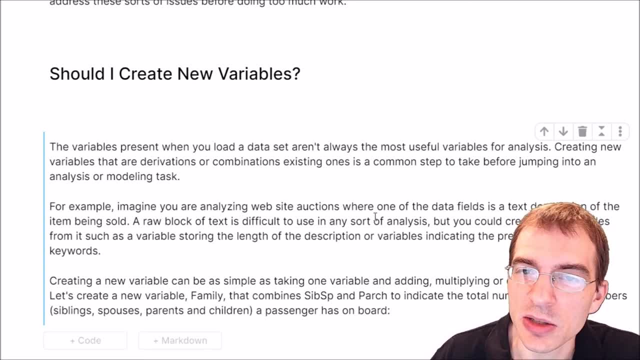 derivations or combinations of the existing ones that you're given is a common step that can help you create some more useful information for whatever task you're working on. This process of creating new variables is known as feature engineering. Now, creating a new variable can be as simple as just adding. 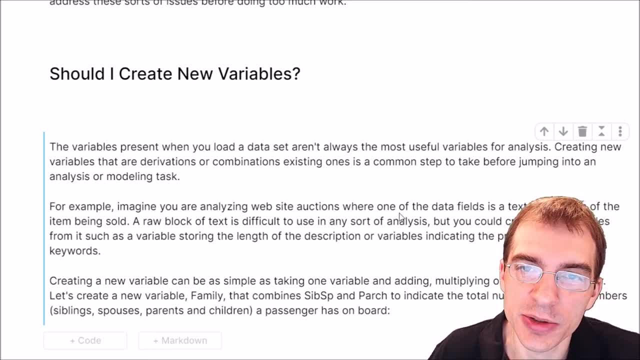 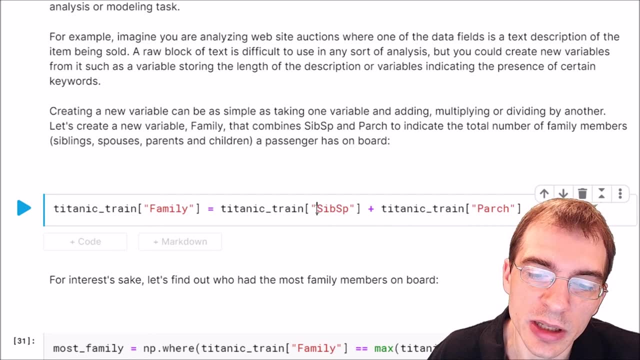 subtracting, multiplying or dividing two numeric variables together. So we'll give an example of how we could do that. So in the data set we had some variables related to family, one that told how many siblings a person had on board and another. 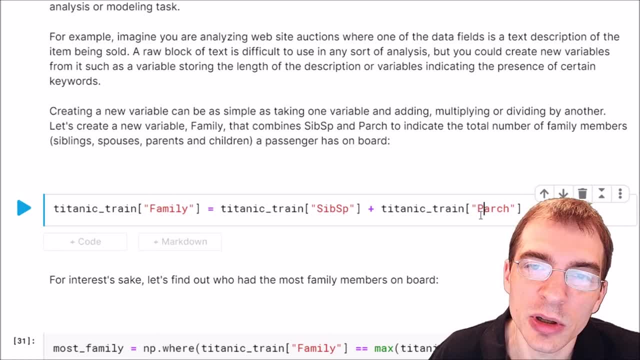 that told how many parents the person had on board. Well, if we added those two things together, it would just be an overall metric that showed how many family members they had on board. So we could easily create a new variable called family. that's just the sum of those two things. 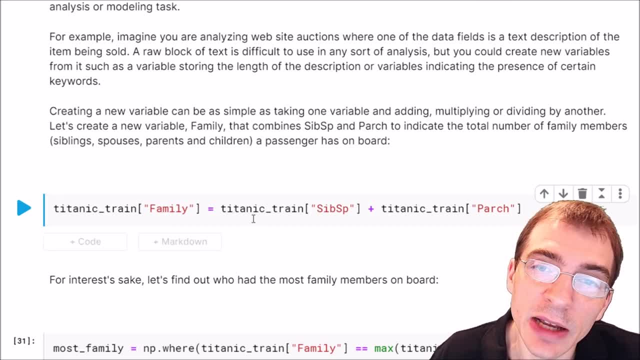 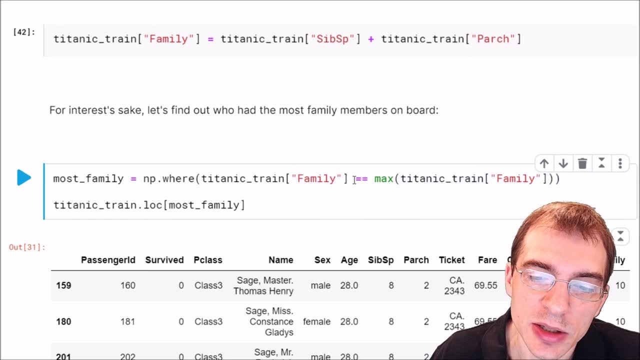 So we'll run that to create a family variable And now that we have that, for interest sake let's see who had the most family on board. So to do that, we can take our new variable family check where it is equal to the max of itself. 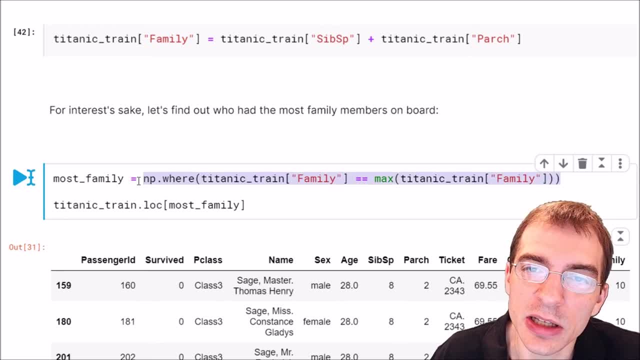 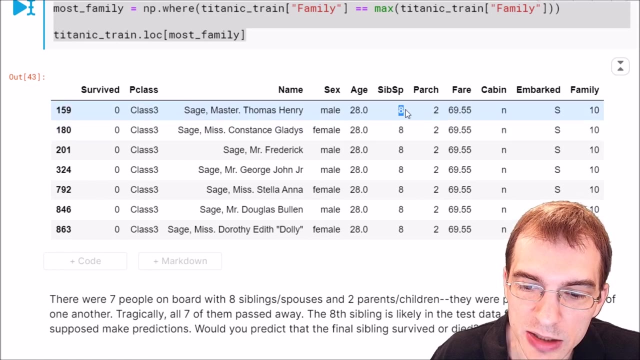 and run npwhere on that whole thing to find the indices where that is true, Then we can take these indices to index back into the data set to extract those records. When we run that we can see that there are several people actually that had ten family members on board and that had eight siblings on board. 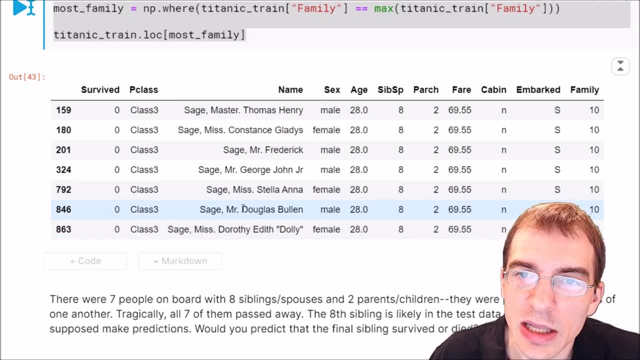 So all of these different people were actually siblings of each other And sadly, all seven of these siblings have been listed under the survive column. So that means none of these siblings survived the Titanic disaster. So to wrap up, in this lesson we covered several general questions. 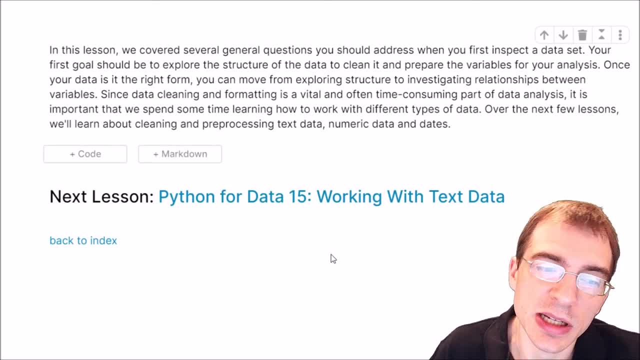 that you should think about addressing when you first inspect a data set. Your first goal when you load in some data is to explore its structure and then prepare the variables for your analysis only after you have cleaned the data and gotten it into a format that you can work with. 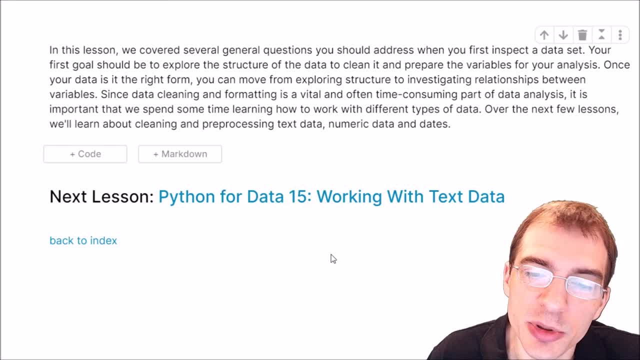 Can you move on and do more complicated analyses and prediction tasks? Since data cleaning and formatting is a very important and often time consuming part of data analysis, it's important that we spend some time learning how to work with different types of data and how to manipulate data better. 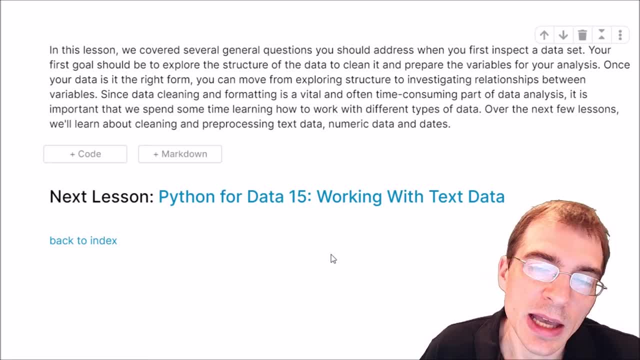 So over the next few lessons we'll go more in depth as to how to clean and preprocess different sorts of data, including text data, numeric data and dates. If you found this video useful, you can drop a like, hit subscribe, and I will see you again next time.